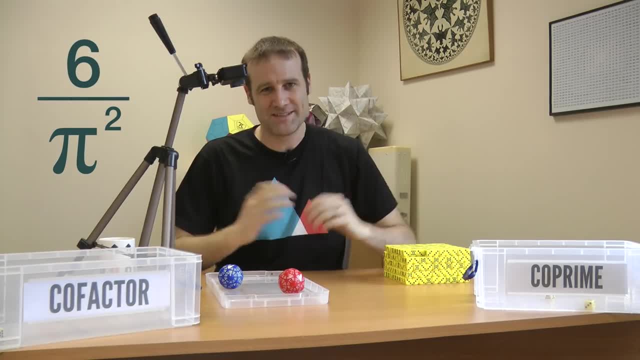 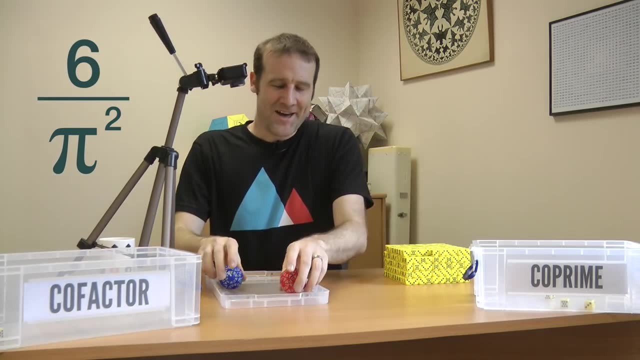 I love the fact you're doing some seemingly unrelated bit of math and once again pi shows up. Uh, 1.. Oh, okay, 1 and 38.. That's pretty straightforward. Now, this unexpected appearance of pi in the probability of random numbers being co-prime. 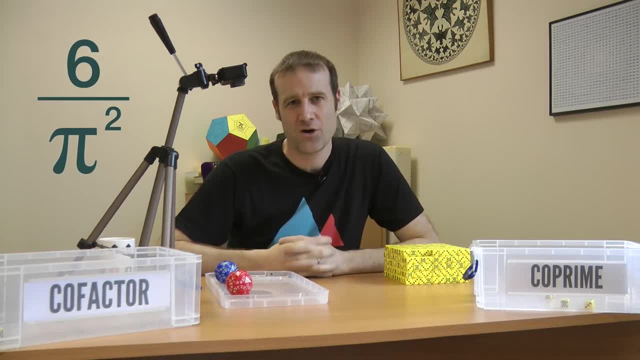 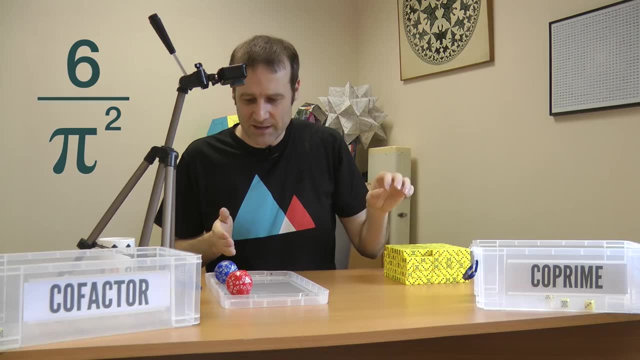 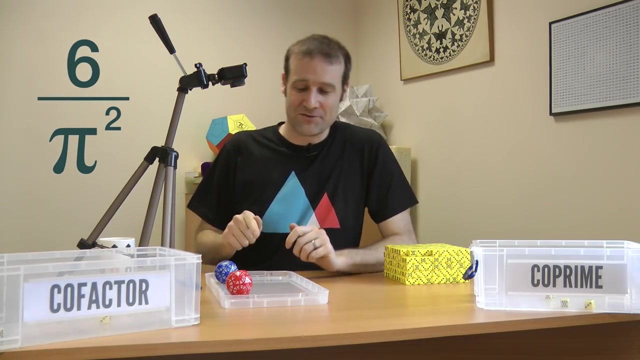 means that I can calculate pi in possibly the most convoluted, ridiculous way I've done yet. So I'm going to experimentally work out 111 and 114,, both divisible by 3.. There you are, By rolling these over and over and over again. I'm going to roll them 500 times. 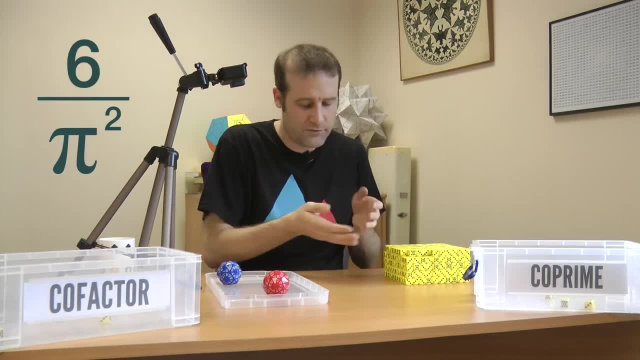 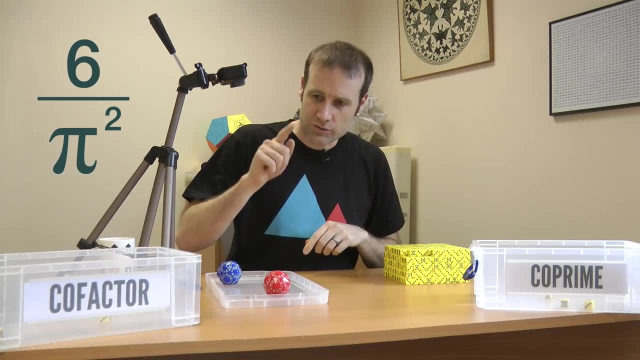 I'm going to keep track of that with. I've got 500 dice, so they're not involved in generating the random numbers. These are just tokens and each time I roll them together I can put the next one in, either co-prime or co-factor. 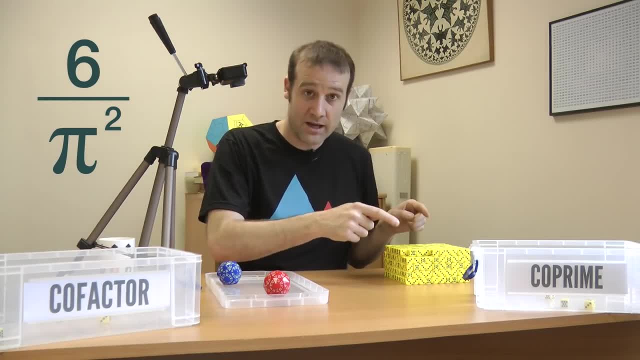 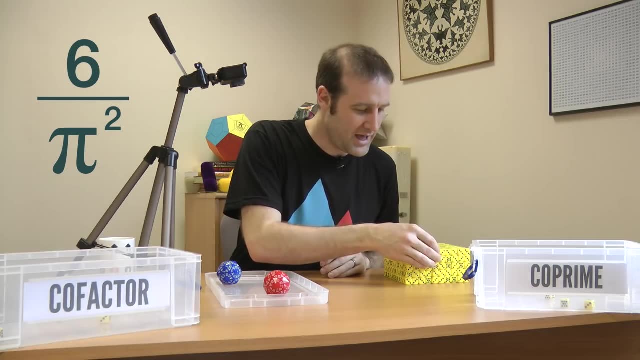 I know I've got 500, because I've arranged them in a 10 by 10 by 5.. So I'm going to do a cuboid At the end of doing all of this. uh, 34 and 98, I will have a rough approximation of the probability of two numbers being co-prime. 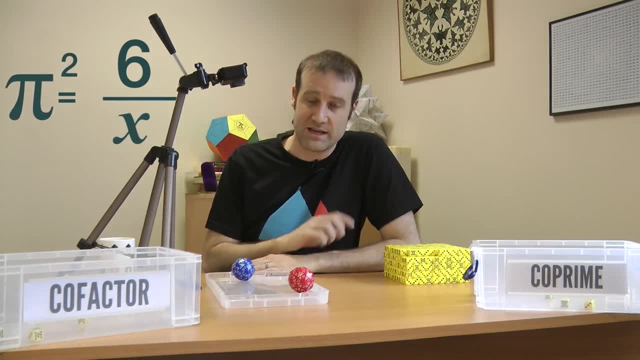 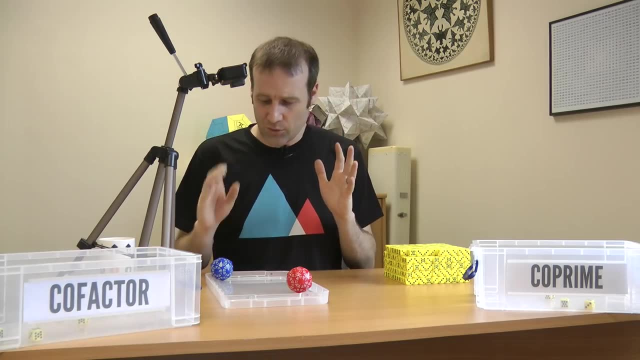 I can then get 6, divide it by that probability, take the square root and I will get pi. I mean, how could this possibly go wrong? So that you know it's all um above board and I'm not doing both. divisible by 3, I'm not doing anything sneaky. 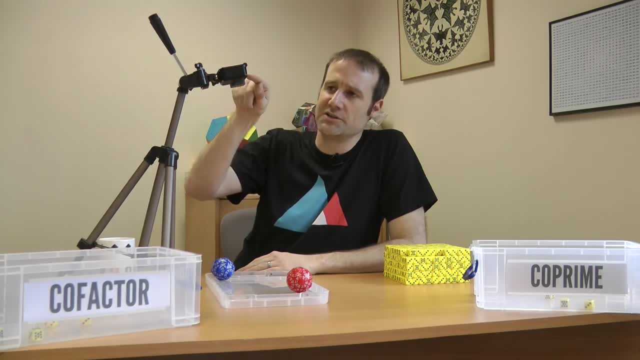 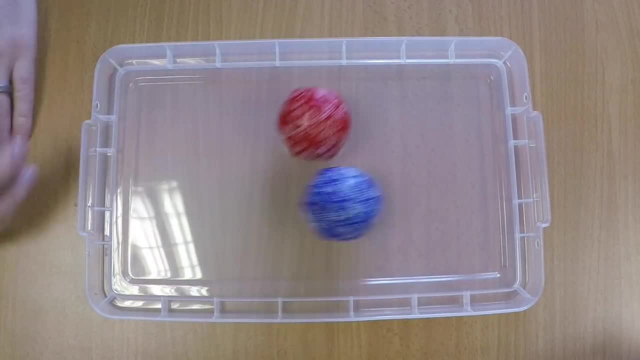 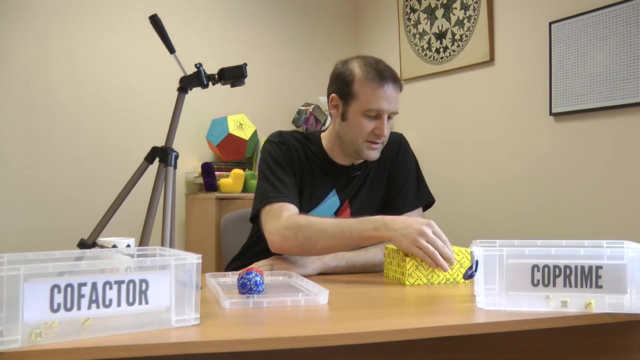 I have this kind of obnoxious GoPro right in the middle, So I will be able to release the complete footage of me doing all 500 rolls. I'm already regretting this. I've only done the first 7, and I've realized what a terrible idea this is. 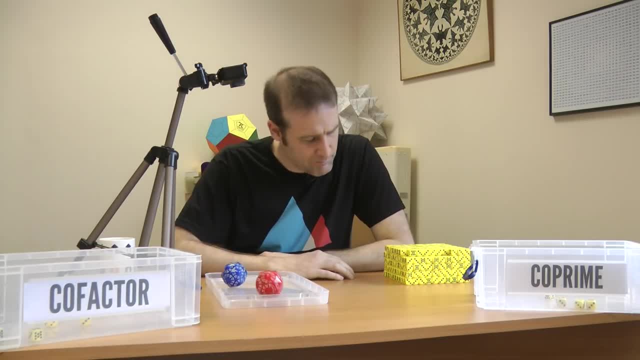 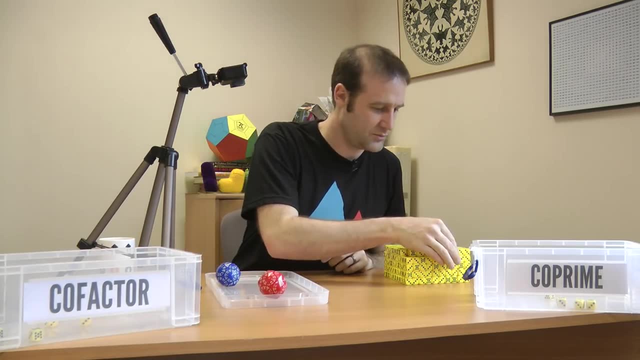 So, uh, I'm going to carry on for a while. I'm probably going to get bored. I'll get 100 or so in and then I'll stop for a break. uh, 93 and 12. And I will show you the proof of how we know the probability. 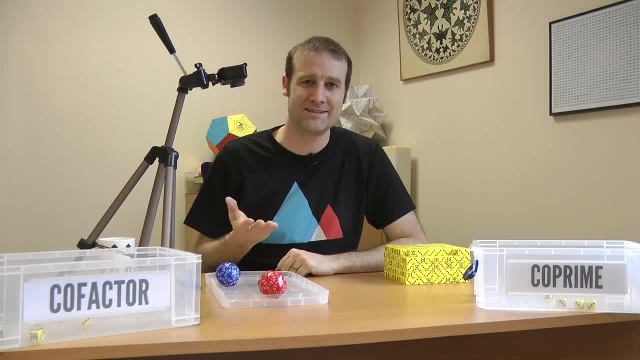 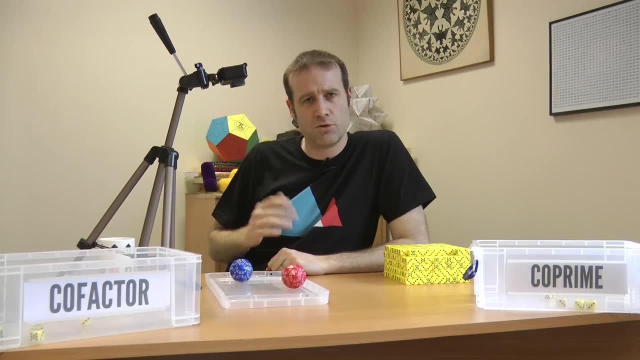 The probability of two random numbers being uh. co-prime is 6 divided by pi squared. So you get to enjoy me doing this now in more of a montage fashion. I'll well, a much more exhausted version of me will be back with you in a second. 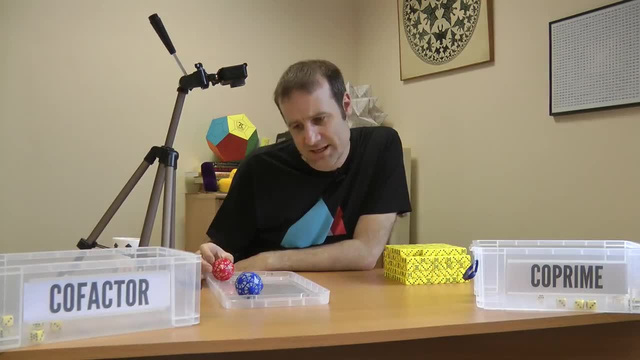 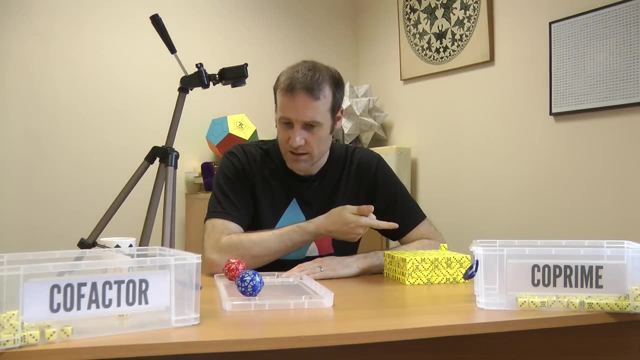 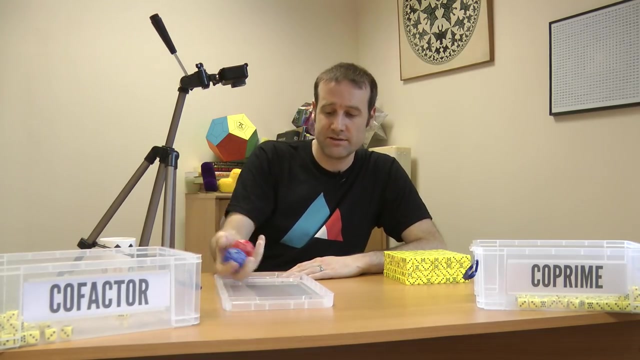 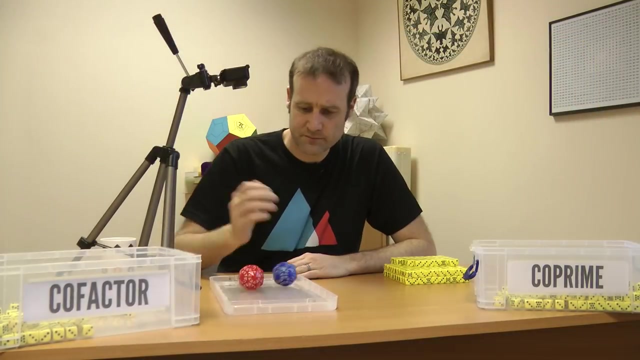 21.. Oh my goodness, I've almost done a layer. 113, that's prime, What a way to go out. And 41. There you are, double prime, And the 250th roll is 169, which is a great score in darts. 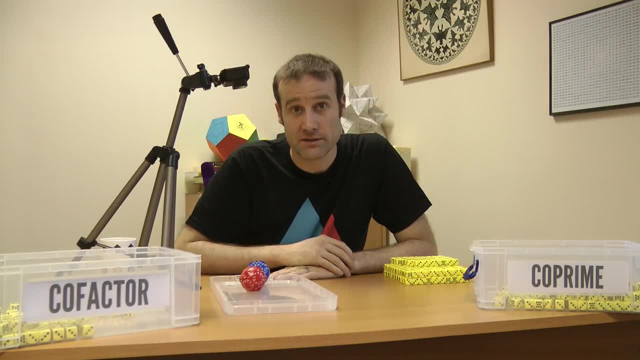 And uh, if you've watched the very long version of this, uh, that is a hilarious callback. And uh, 100 is only got 5s and 2s. 69 has not got anything. So either they are co-prime. 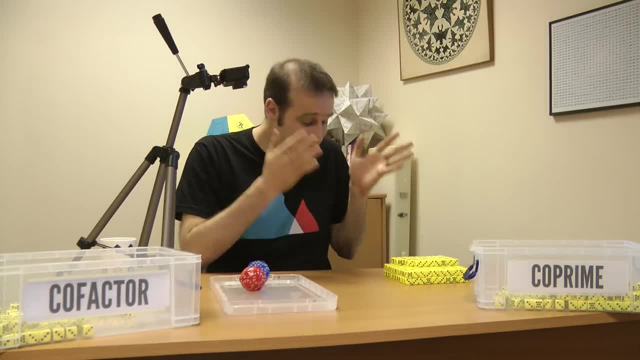 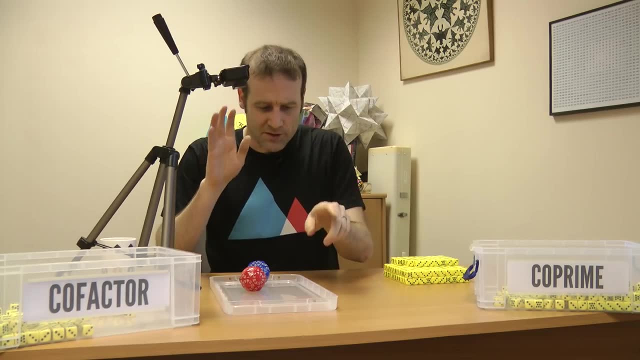 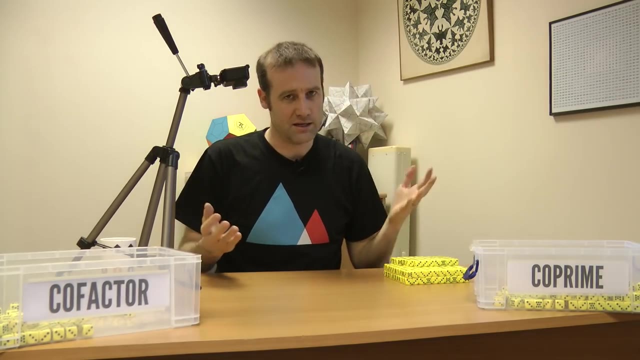 Okay, so I am halfway through. I've done 250 of these for my own sanity And in terms of the mathematical content of this video, I'm going to stop here for a second And I'm going to show you a- uh, a fairly good proof of why the probability of two random numbers being co-prime is 6 divided by pi squared. 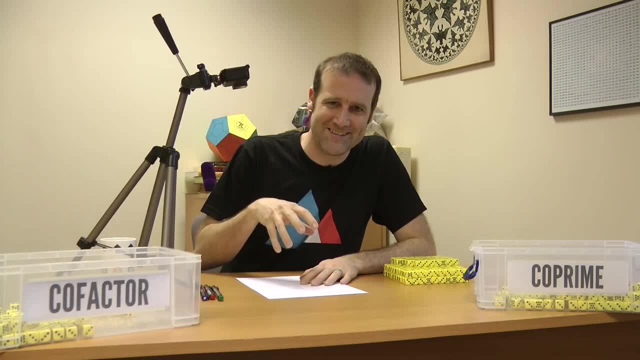 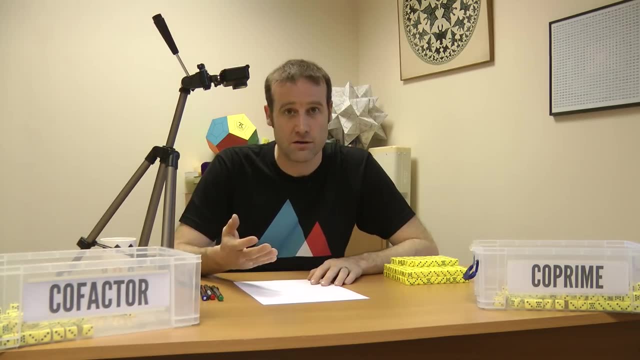 I say fairly good, I'm not going to write it down as rigorously as you could. In fact, I will have a link in the description to a few different proofs for this same thing that involve different amounts of previous knowledge. This one is just my favorite one, I guess. 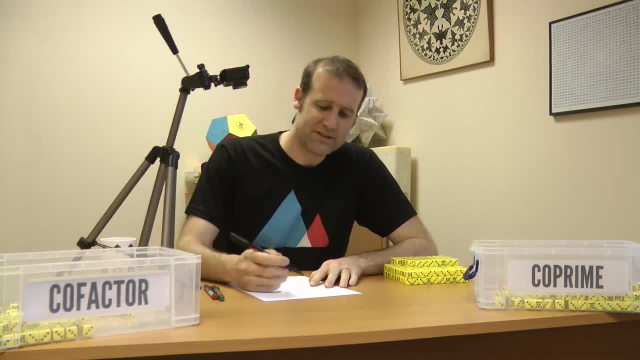 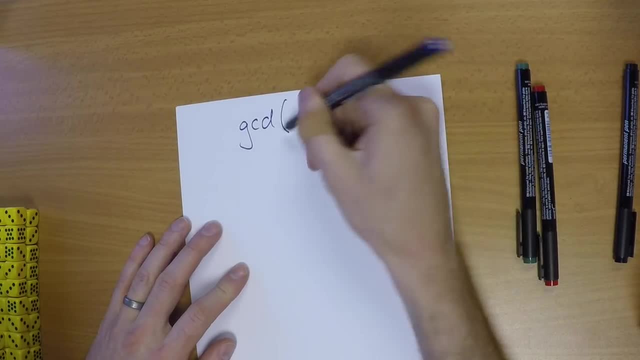 So, notation-wise, what we're saying is: if you want to find the um, the greatest common denominator of two numbers, Uh, so you've got two numbers: m and n. I'm going to write down the gcd of n. 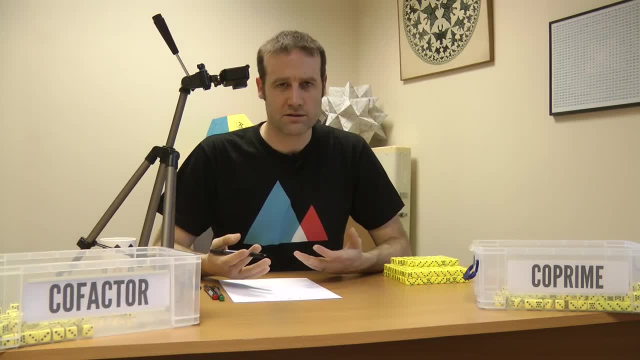 The gcd of m and n. that just means what is the greatest common denominator. So if m and n were co-prime, you would get uh one out the other side. And then the last bit of notation is in terms of probability, is uh the probability of something? 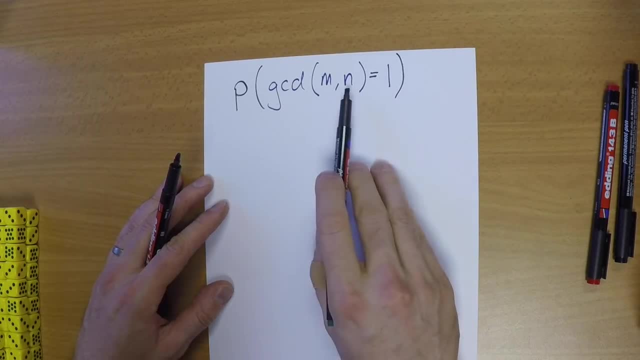 I'm going to put it in brackets like that. So the probability of uh two numbers picked at random having the greatest common denominator of one- In other words they're co-prime- Uh equals. that's what we're trying to work out. 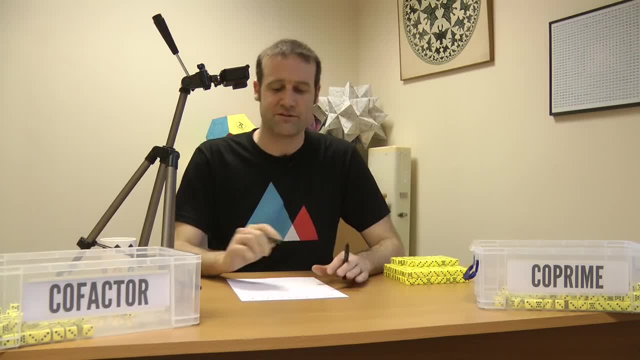 And I'm just going to call that x for now. right, So that that's what we're trying to find. What? what is that probability? I'm going to name it x. I'm going to now set up a semi-related situation that will then incorporate x. 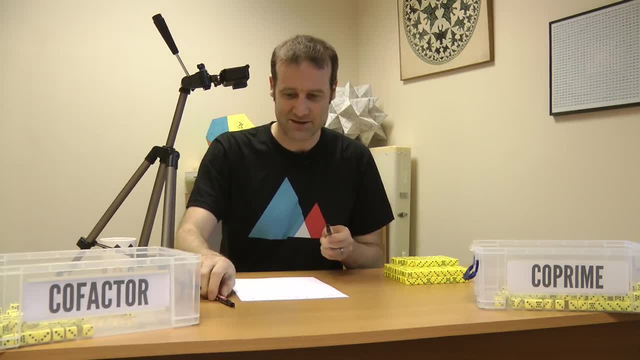 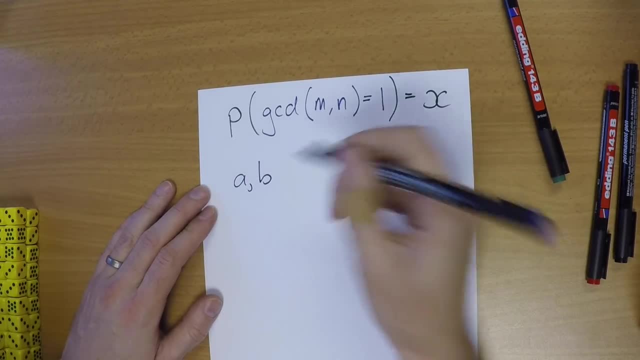 We rearrange it and we can get x out- uh, the other side- with a value attached to it. So the situation I'm going to set up is you've got two numbers, a and b. They're both integers. You've then got some random number k, another integer, which is smaller than both of them. 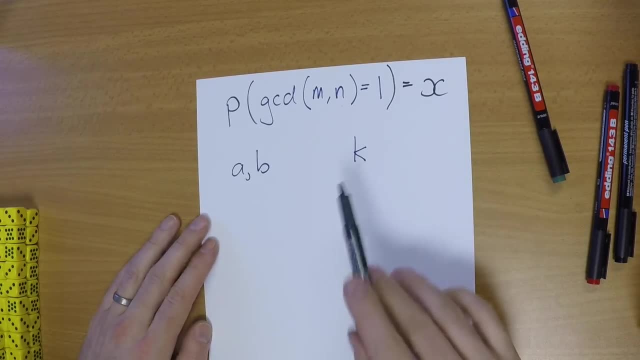 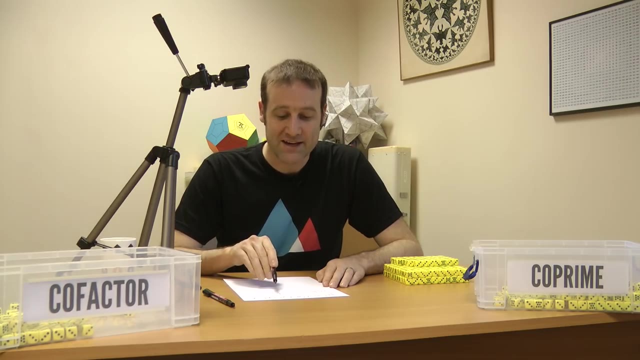 This is the hand-wavy bit, So I'm going to ask the semi-related question: if I pick two integers at random and then an integer smaller than them, what is the probability that k is the greatest common denominator of, uh, those two? 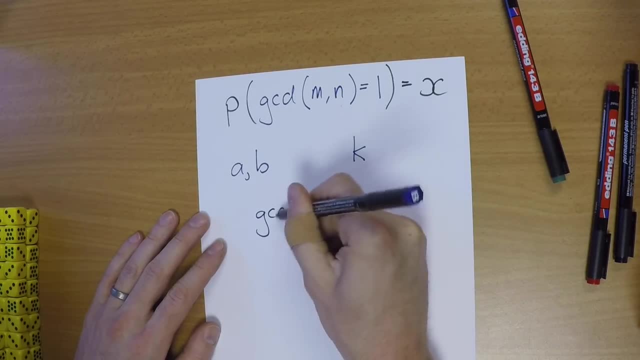 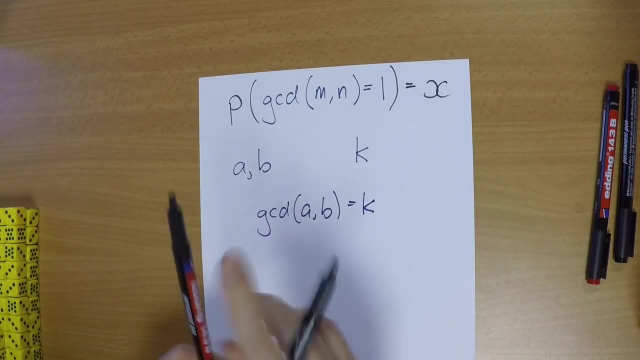 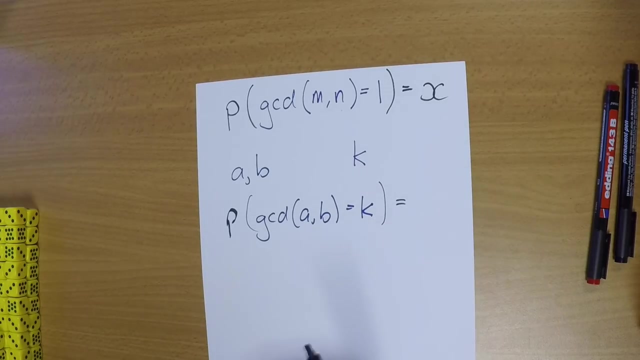 I want to find out the greatest common denominator of a and b, equaling k or, more to the point, I want to know what is the probability that the greatest common denominator of a and b is k. Well, k has to divide a and b, right. 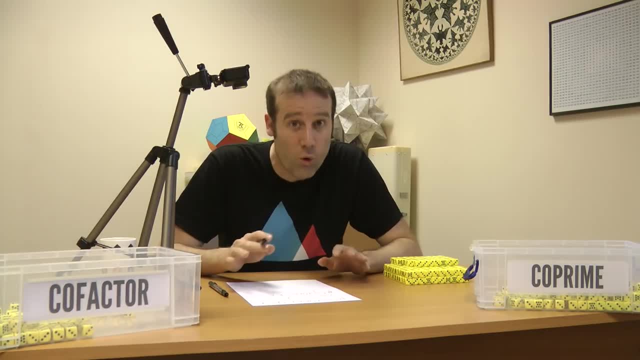 For it to be a denominator or, you know, a factor at all, it has to go into both of them. Well, if you think about it, two goes into a half of all numbers. Three divides into a third of all numbers. 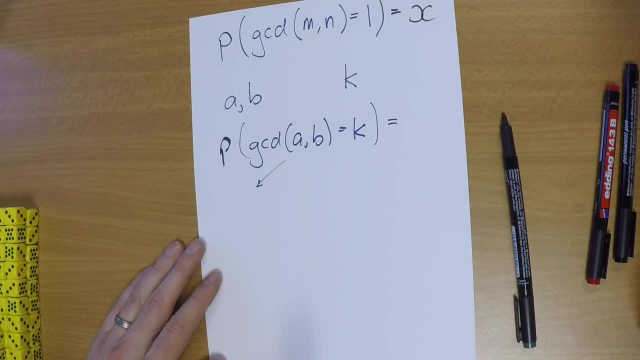 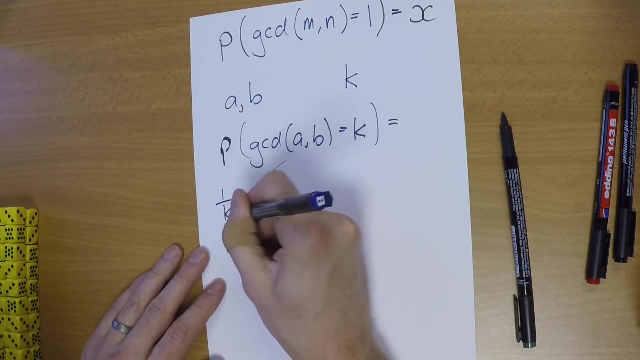 Four divides into a fourth of all numbers. K divides into a kth, one over k of all numbers. So actually the probability of it dividing a perfectly evenly is one over k. The probability of it dividing b perfectly is one over k. If we want to divide a and divide b, we multiply it together. 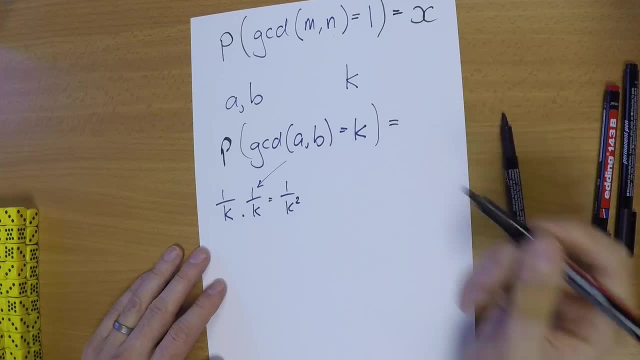 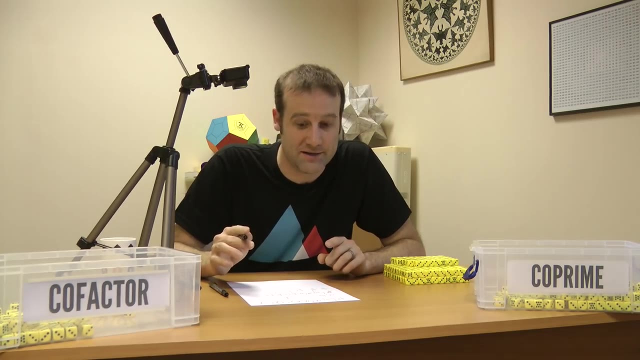 It's, uh, one over k Square. Okay, that's all well and good, Uh, secondly, what else do we need? Well, for k to be the greatest common denominator, there needs to be no other denominators that go into it. 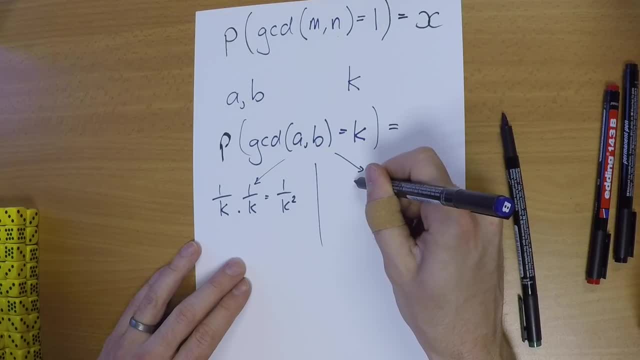 Because then we could just multiply them together to get a bigger factor that would go into it. So if you've got a already divided by k, you've got b already divided by k, what is the probability that that greatest common denominator is one? 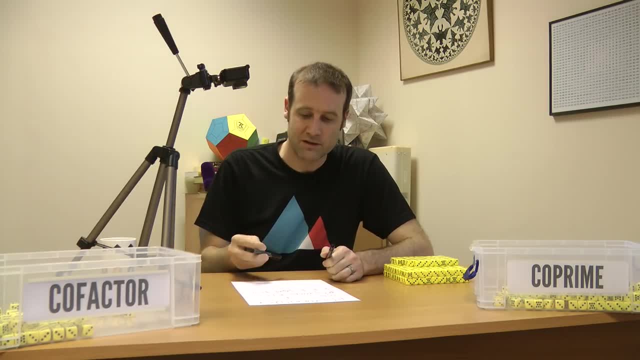 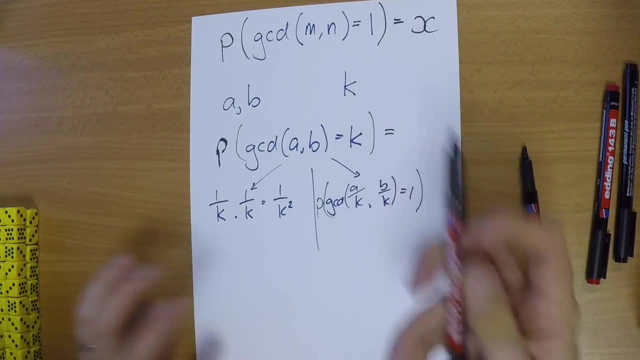 So we're asking: what's the probability of that? And oh, wait a minute. We've already specified: the probability of two whole numbers having a greatest common denominator of one is equal to x. So actually we know that That just equals x. 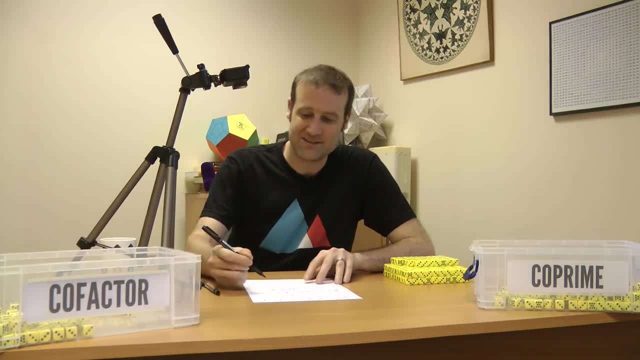 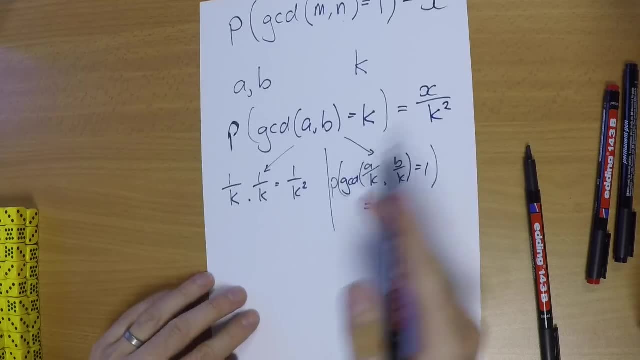 And for this to be true, we need to have this and this. So it actually equals x divided by k squared, And you go okay. well, that's all lovely. Now we know the probability of picking k is the greatest common denominator is x divided by k squared. 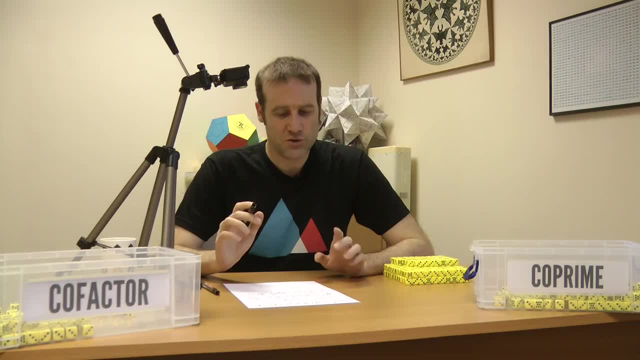 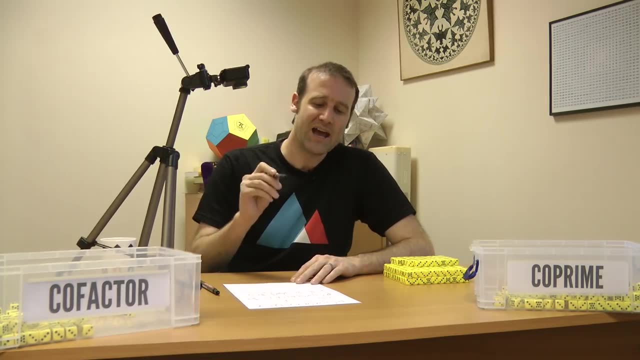 So what? Well, here's the thing: Two numbers have to have a greatest common denominator. It can be one, but it could be bigger, But there has to be one. And so if you were to add up, so for a and b, if you were to add up the probability of it being one, 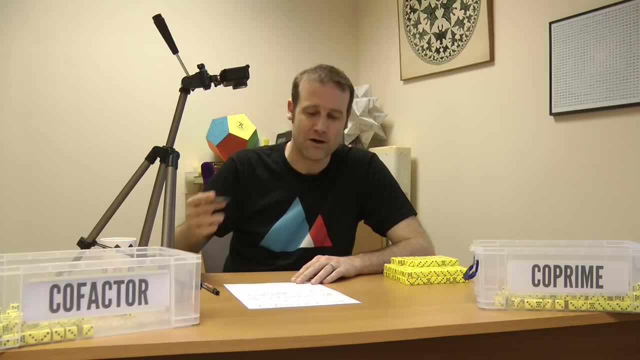 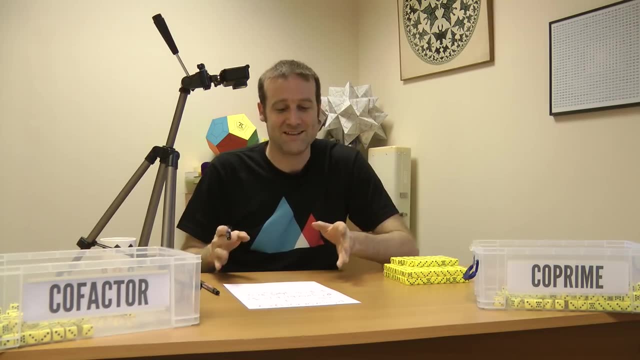 plus the probability of it being two, plus the probability of it being three, plus four plus five, all the way up to whichever one is the smallest, and you add them all together, there has to be one, And so the probability has to equal one. 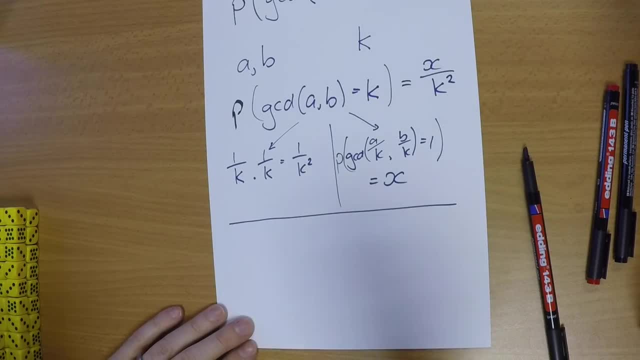 So if you add all the probabilities, you should get a total of one. Which is to say, if you were to sum up, every single x divided by k, squared, starting with k, equals one, all the way up to however big these numbers are. 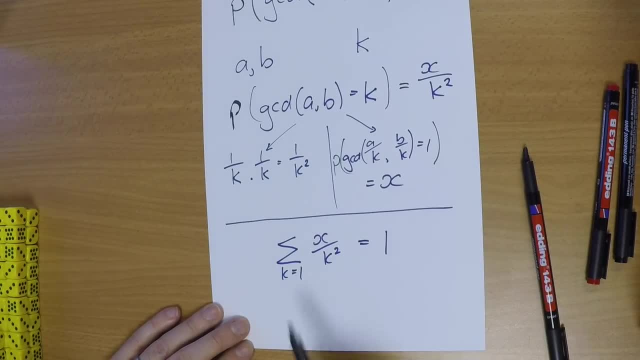 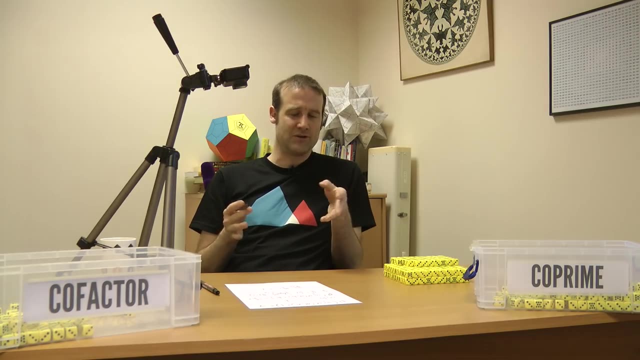 that total sum has to equal one. And well, how far do we have to sum? Well, here's the thing: I've been a little lazy when I talk about two random numbers, Because if you just say two random numbers and you don't put an upper bound on it, 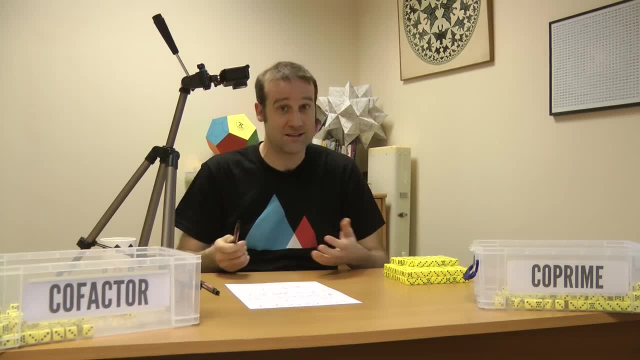 they could be arbitrarily large. You could have some massive numbers. In fact, statistically they're going to be big, Most numbers are, So I've been doing this with d120s, right, So there's only 120 sides. I've been picking from a tiny, tiny section of all possible integers. 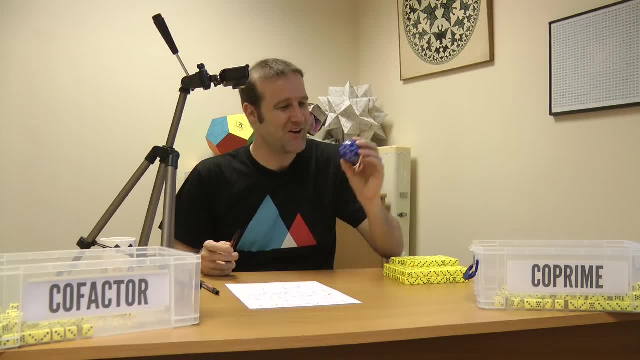 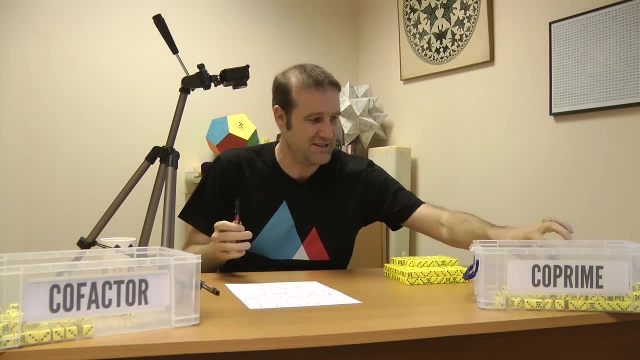 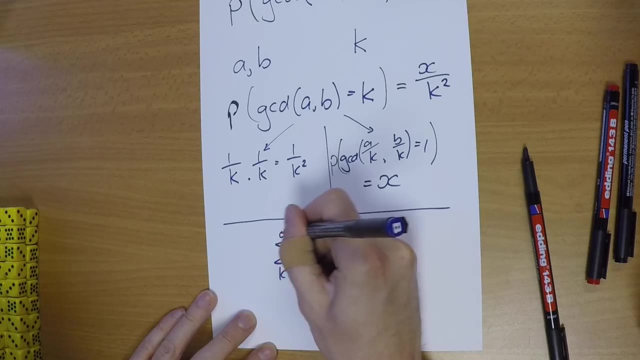 That may be the greatest understatement I've ever put in one of my videos. So in the true limit right, in the real absolute max situation, this can be arbitrarily large, right, This will tend to infinity. So just for argument's sake, let's go all the way up to k equals infinity. 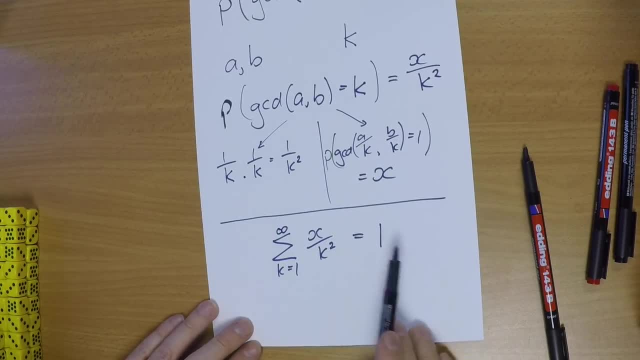 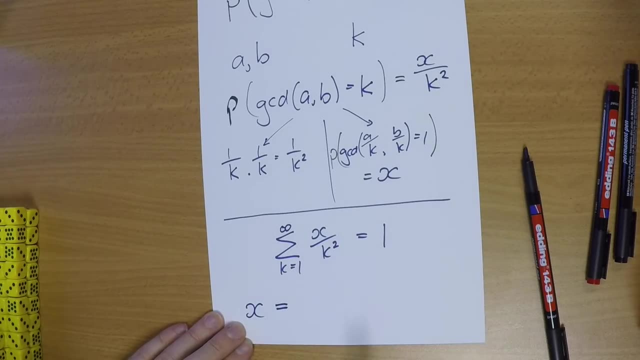 to get the correct answer, And so we now know this holds. We can do a little bit of rearranging. We want to find x, So we know that x equals well if, because x is a constant, we can bring it out the front over here. 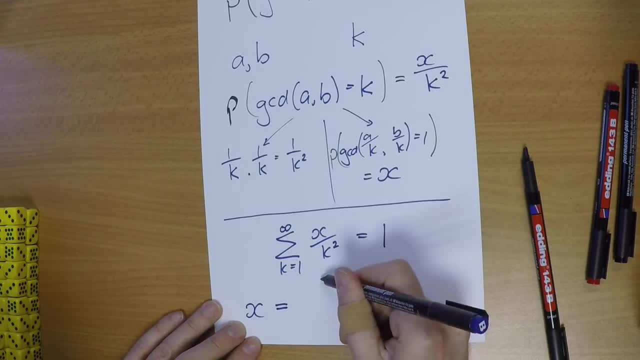 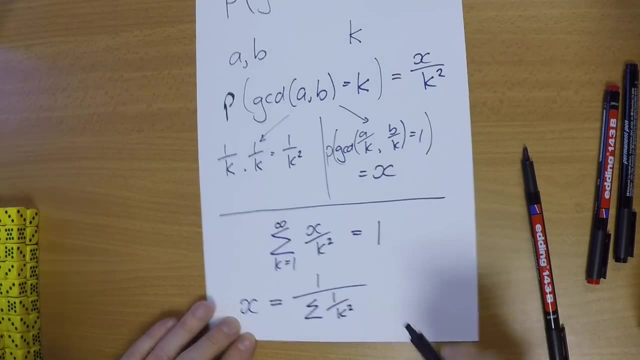 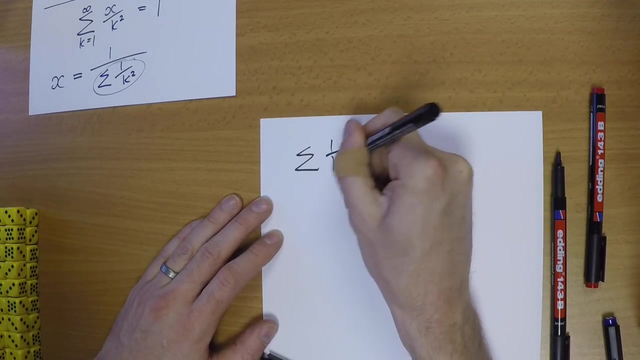 We can then divide both sides by that. x equals the inverse, It equals one over the sum of all sides. So that's k squared fractions, And I'm going to break out onto a second piece of paper here If you want to work out the sum of all k squareds that equal. 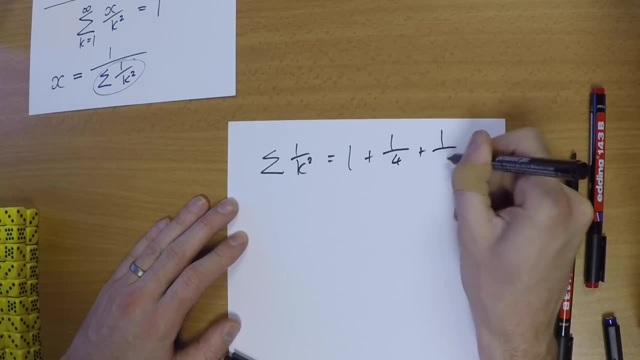 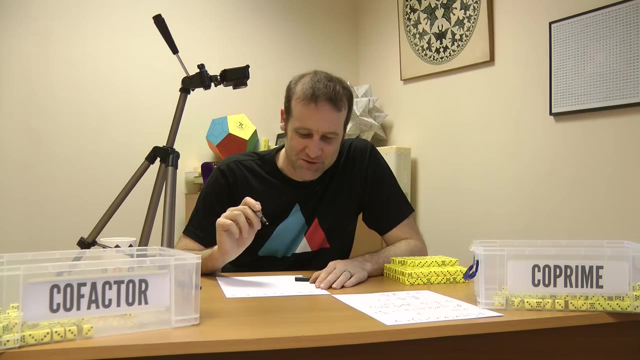 well, that's 1 plus 1 over 4, plus 1 over 9, plus 1 over 16.. And you keep going all the way up. dot dot dot. So this is actually called the Basel problem, And Euler was the first person to solve this. 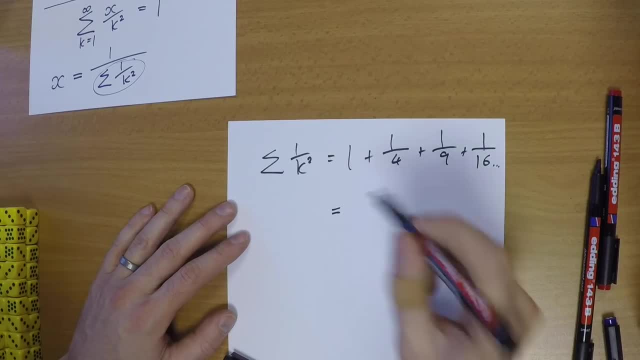 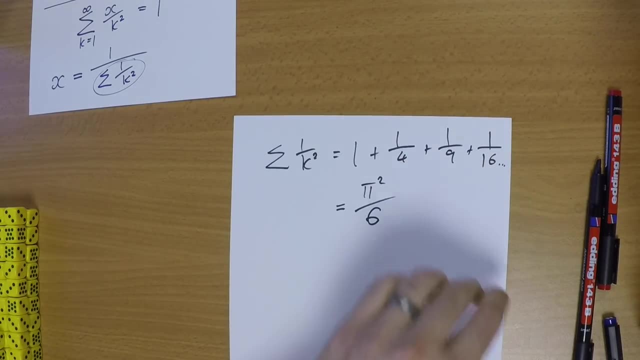 and he was able to prove that limit equals if there are infinitely many of these pi squared on 6, which is why I can then say that x, our original probability we were looking for, is equal to 1 over pi squared on 6,. 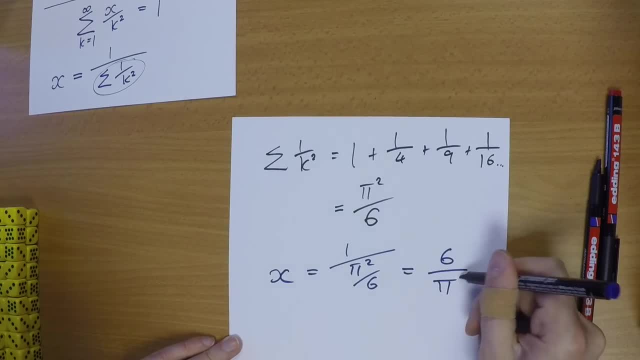 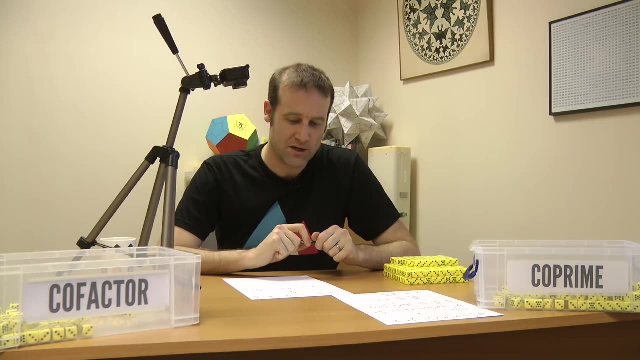 which, of course, is just 6 divided by pi squared, And that's where it comes from. At this point I will accept it's a little bit unsatisfying, because I've said pi comes out of 6, I've said pi comes out of nowhere. 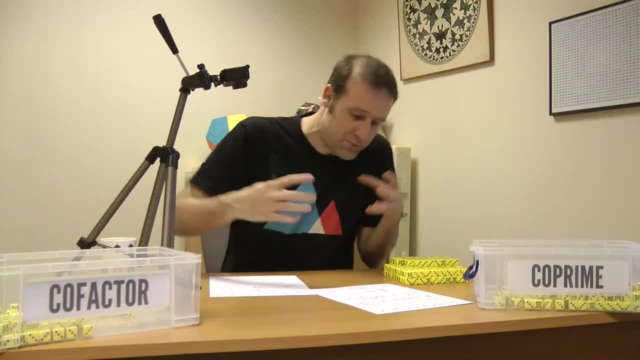 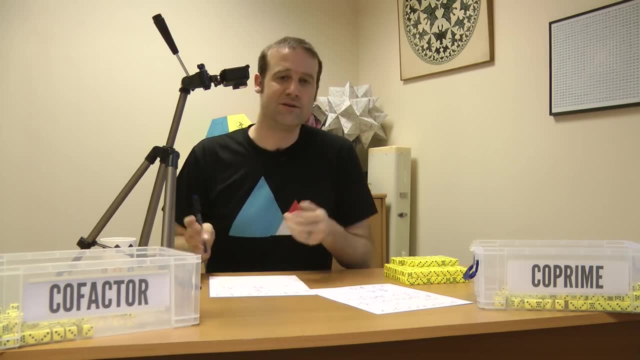 I've done some nice rearranging, a good bit of logic. I've managed to corner the probability, rope it in with this other situation, squeeze out an infinite series for it, and then I've just said: oh, the limit of that happens to be this. 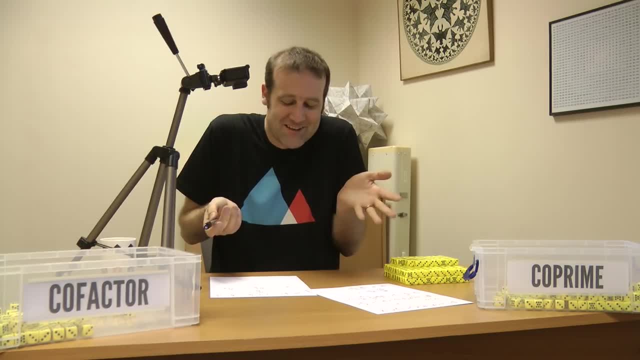 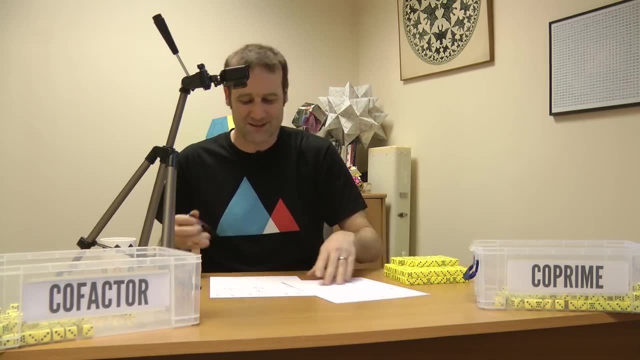 I'm sneaking in the pi here when no one's looking. I mean, I think this is amazing. in math, The probability of two numbers being co-prime comes down to the limit of the sum of all fractions squared. I mean, that's just great. 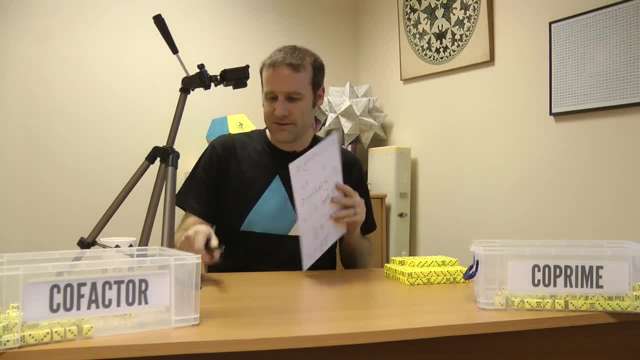 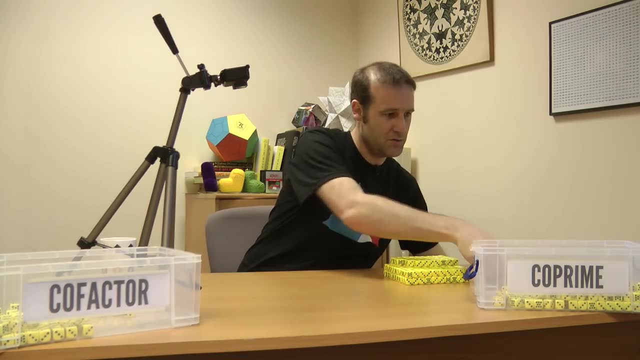 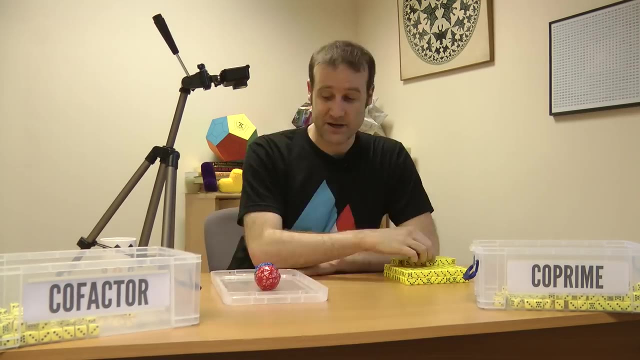 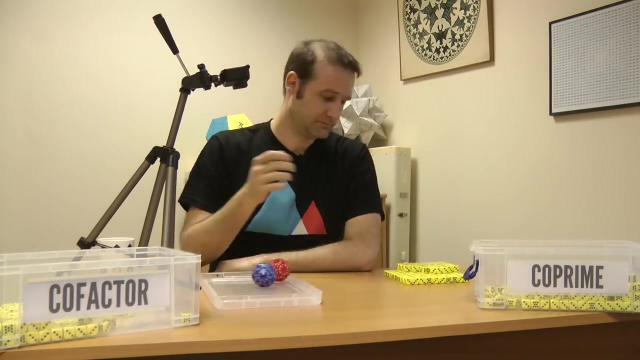 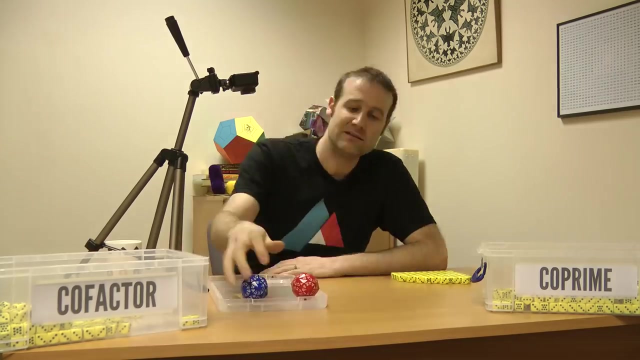 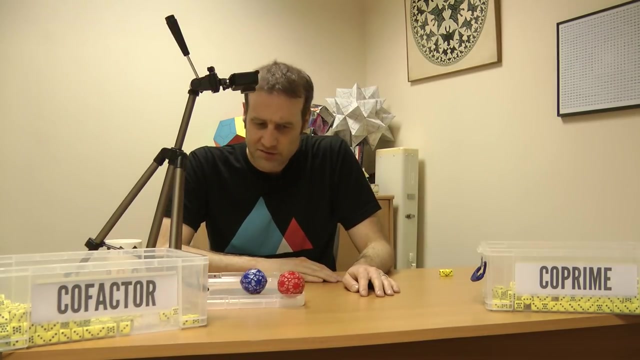 But anyway, enough going on and on about mathematics. It's time to get back down to generating some more random numbers. So here we go, The 251st pair of random. I've just got to double-check everything. I've been making so many mistakes. 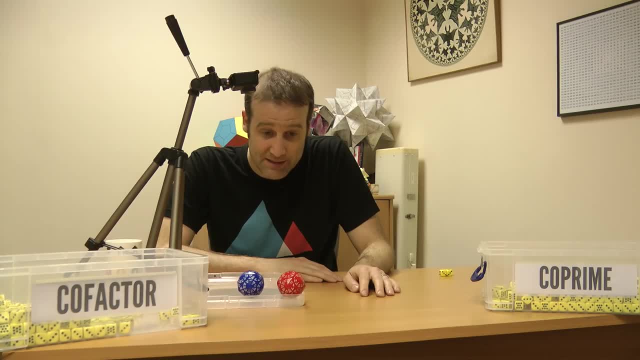 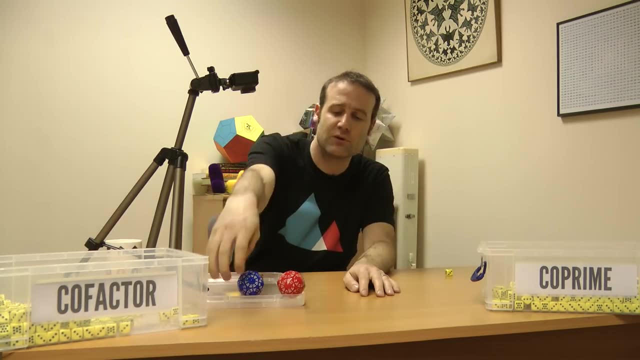 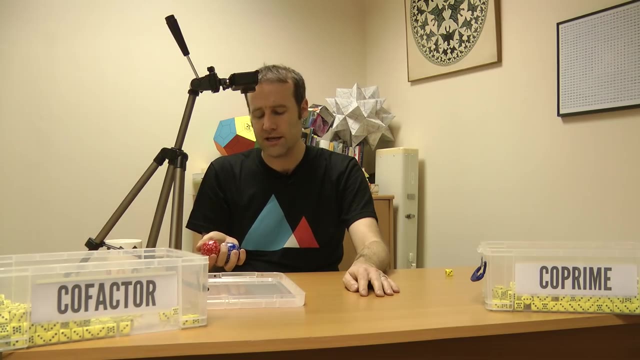 24.. And that's twos and threes, 61.. No twos, no threes. Last roll, last roll. Here it is, Oh my goodness, I have done 998 random numbers, The last two random numbers. 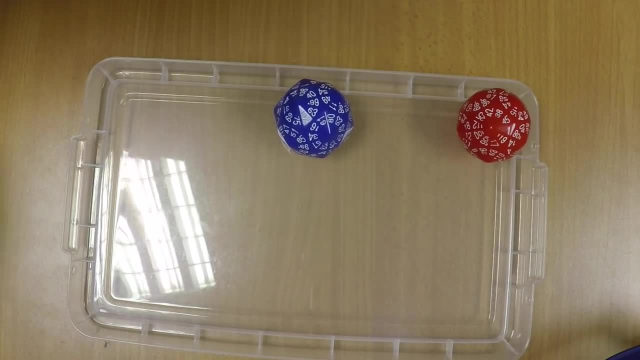 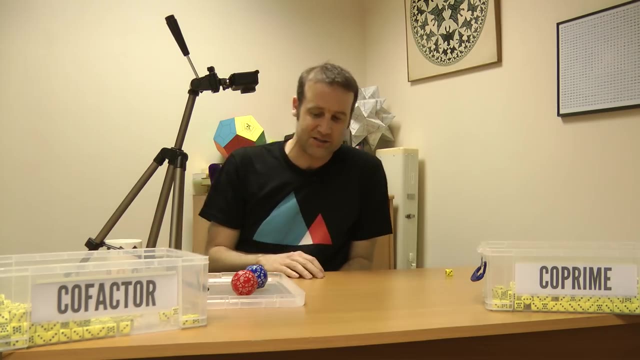 are bringing up to 1,000.. Random numbers are 45,, so that's a three by a three by a five, and 63,, which has a three in it. It's three by 31,, and so they both have three as a co-factor. 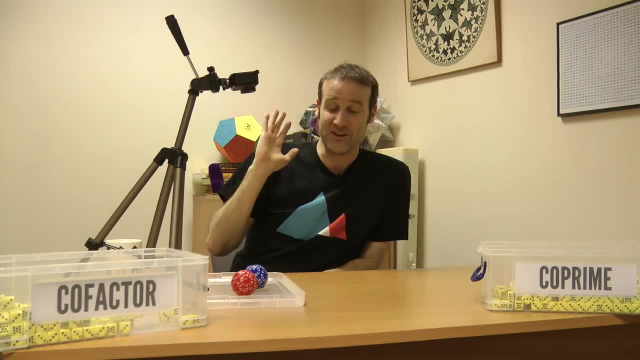 And there you are. It's taken hours And if you want to check the long version of the footage, the link is in the description. You can watch the entire thing, or you can just rely on the fact that enough hardcore pedants watch my videos. 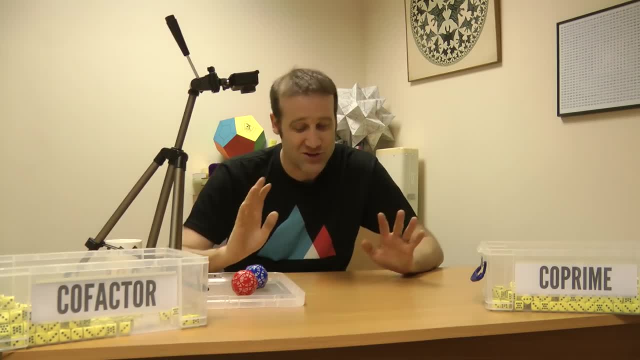 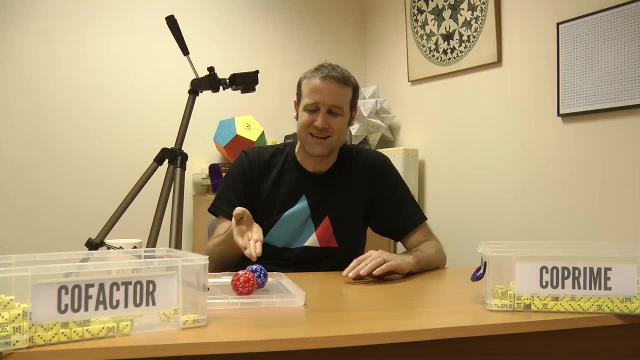 and they will have checked right So you can take Because it's out there. you know it's fine. I've probably made some mistakes. I'm kind of hoping the mistakes have averaged out. So some mistakes. I've not done the co-primality test properly. 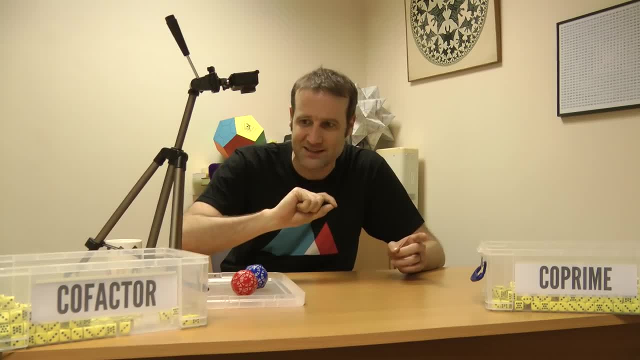 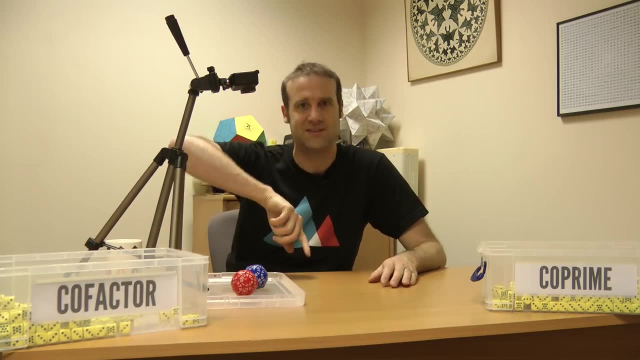 Other times, I swear, a couple times I've just I've instinctively thrown it the wrong way, Who knows? But if you spot a mistake in the long version, let me know and I'll put corrections in the long version of all the points where the mistakes are. 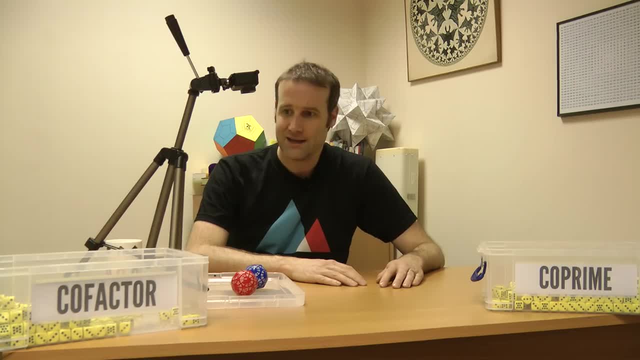 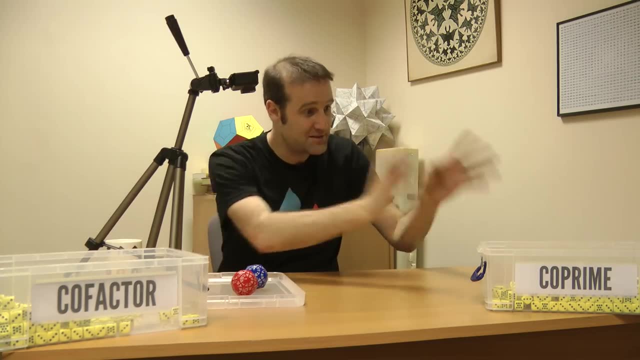 and we'll see if it makes a big difference to the result. And so now, All right, So now we find out if we have pi. So I'm now, I'll count up these, I'll count up these, and then we'll do our final working out. 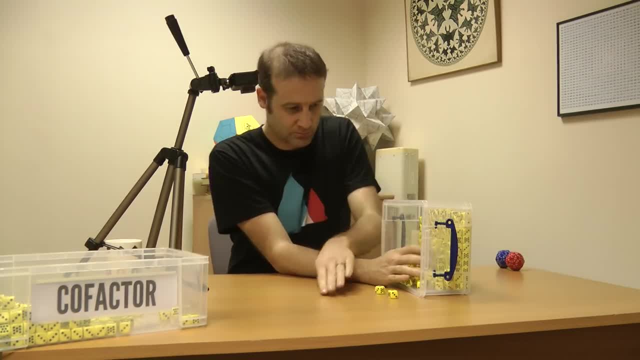 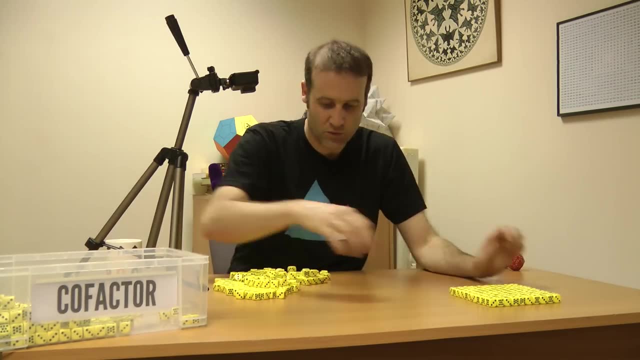 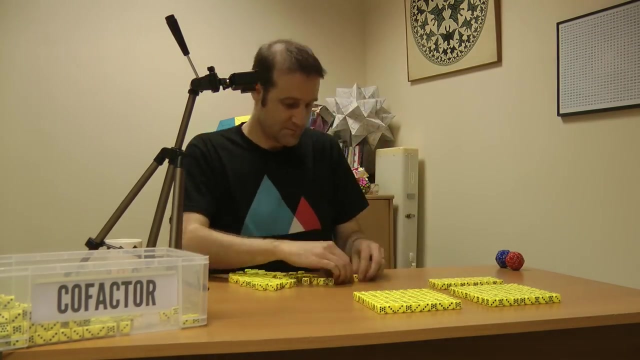 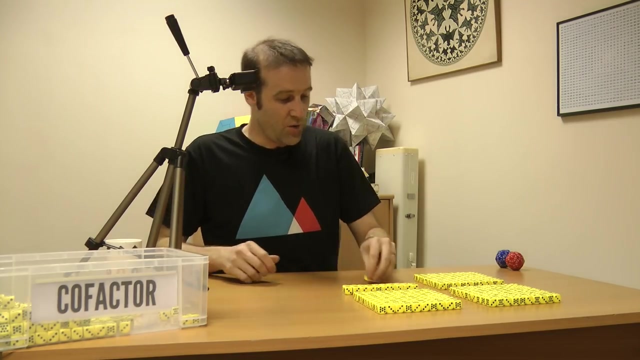 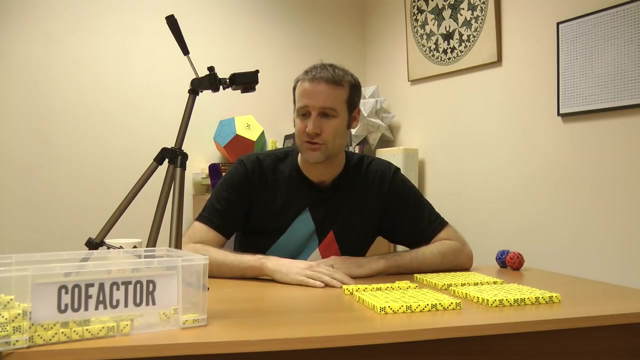 How exciting. Okay, there we are: 100. 300.. All right, 305. 310. 315. 322.. Okay, we have 322 co-primes out of 500.. I could count the co-factors. 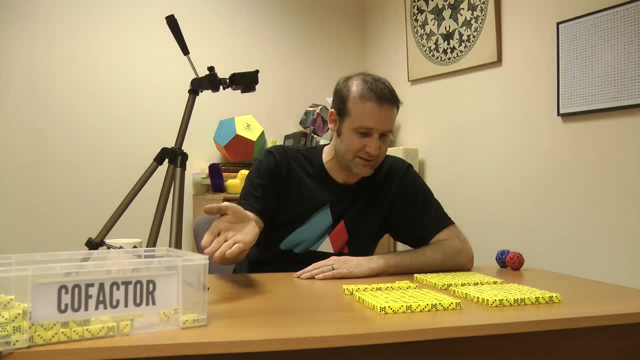 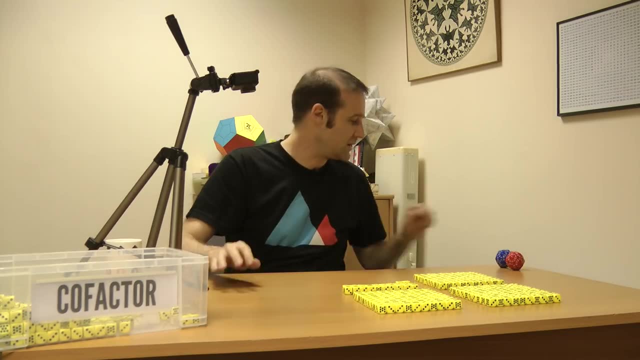 to make sure there are the remaining 178.. I'm not gonna bother doing that, even though it would please me immensely to line them all up neatly as well. I'm too excited, however, to find out how close I got. Like if I'm within 10%. 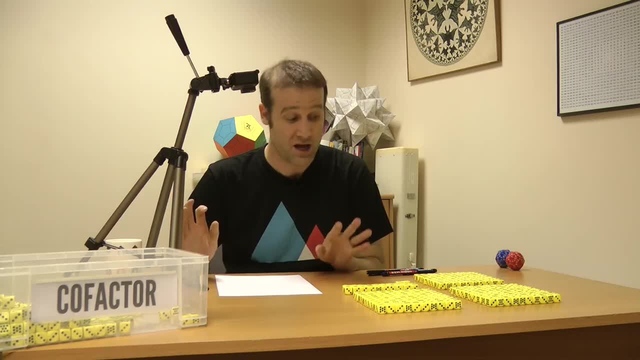 like anything between 3 and 3.3, I will be ecstatic, But I Okay, we'll find out. we'll find out. I guess I'm gonna use my phone- It has a cable coming out of it because I'm using it to record the audio. 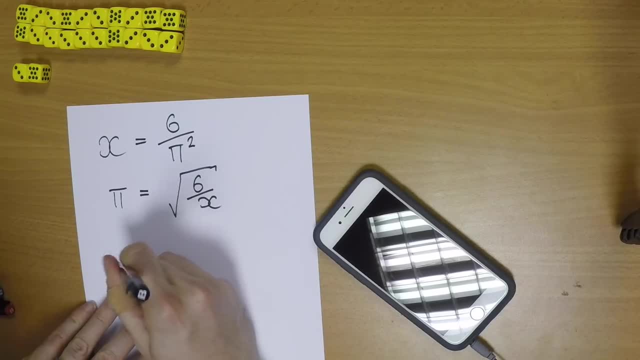 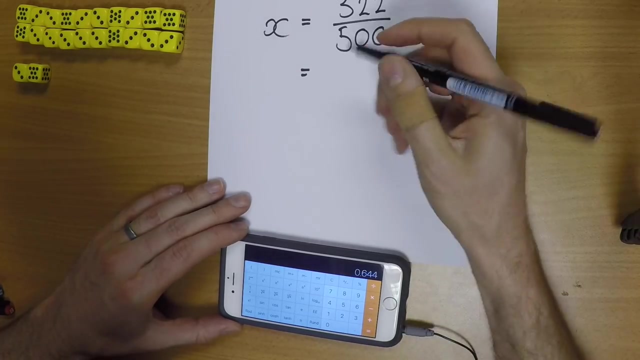 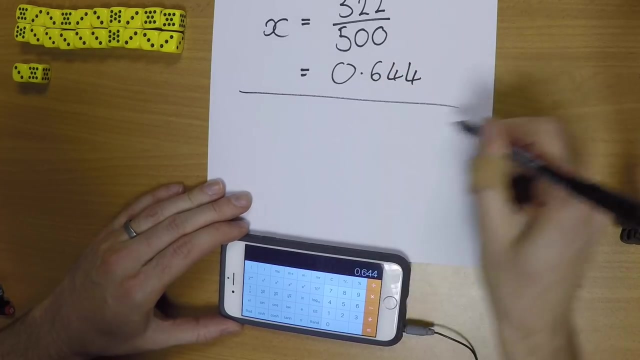 for this video. Okay, right, here we go. Right, so let's do this. I got x experimentally equal to 322, out of 500 equals 322. divided by 500 equals 0.644.. Therefore, pi is approximately equal to. 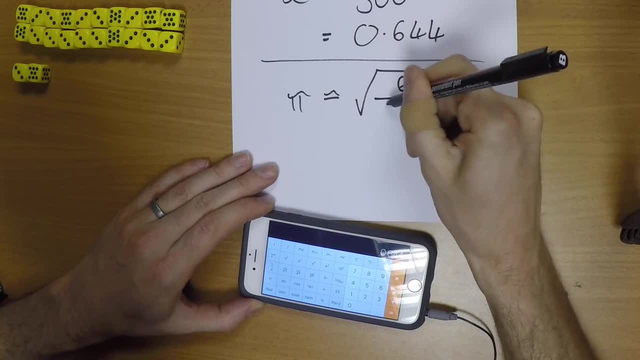 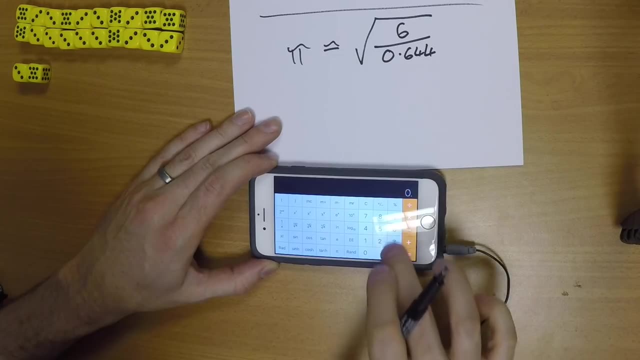 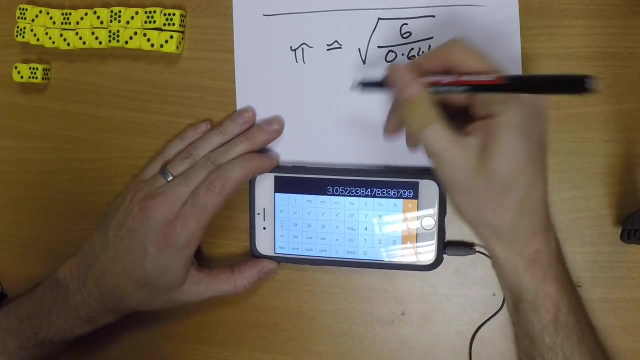 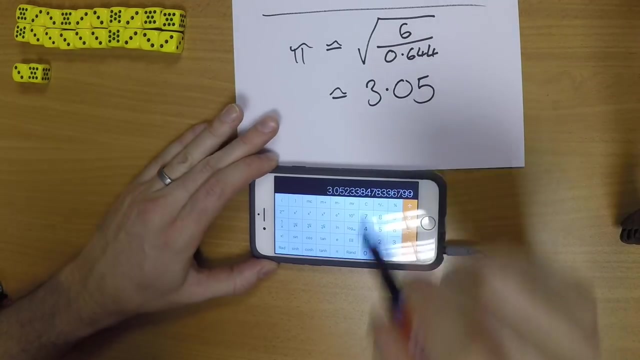 the square root of 6 divided by 0.644.. Here we go. 6 divided by 0.644.. I'm just typing it in instead of using memory or anything. Equals square root 3. 3.05.. Okay, that's fine to be. 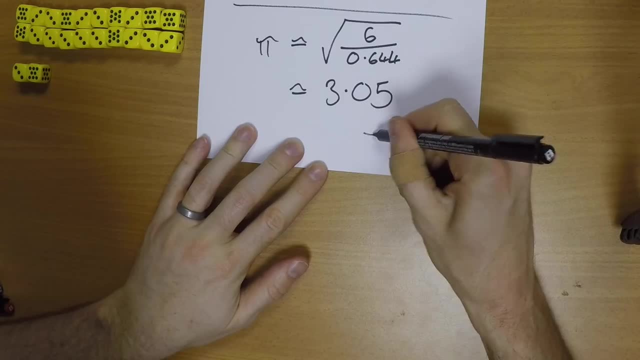 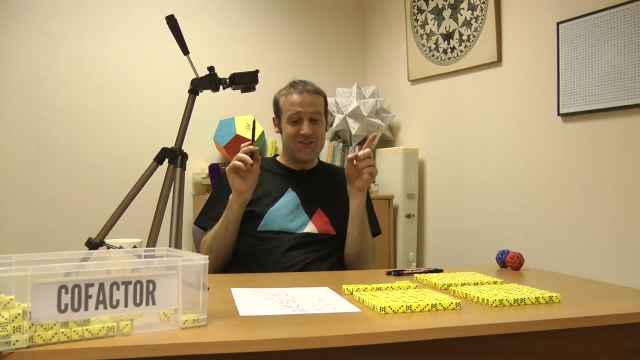 I mean that is only below pi by only 2.8%. I mean that's pretty good. So I admit I did use a calculator at the end to do these working out steps. but I could have done these longhand. 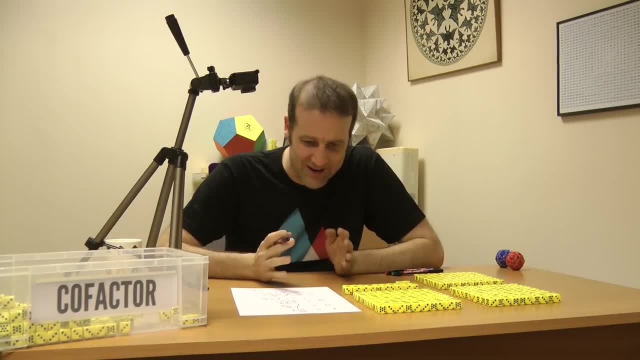 Ignoring that this was a calculation of pi, using solely rolling dice to get random numbers and then counting. Now there are obviously a few mistakes going on, which is why I didn't get super, super close. There are The obvious ones, like 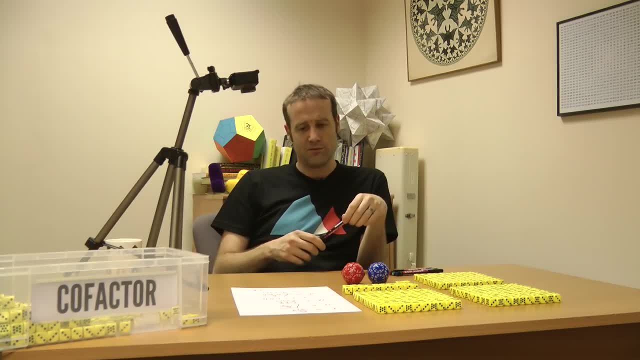 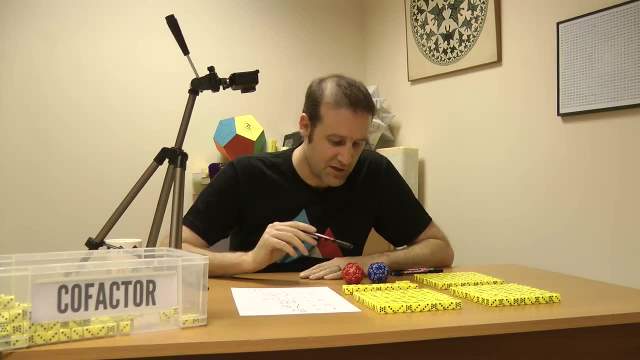 I would have made some mistakes when I was working out what's a co-prime and what's not a co-prime, But the two big things to bear in mind. one of them is that my numbers ended up to 120,, which is pretty good. but in theory, this only works if the numbers you're picking at random can be any size. In fact, they need to be huge, just ridiculously huge, for this to work properly. properly, I worked out if I'm averaging rolls of 60,. 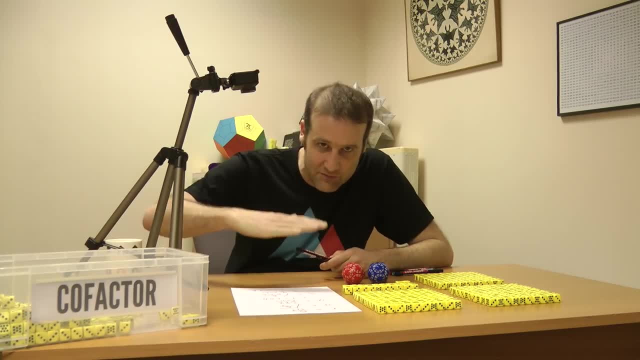 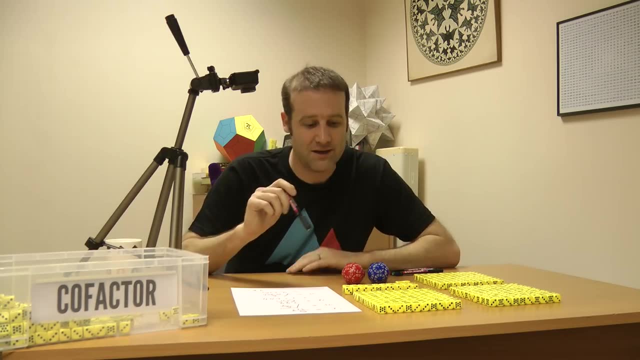 I mean really roughly, it would come out. It comes out under. if your numbers aren't big enough, It would have come out at about 3.12. is the actual value I'm shooting for for pi if you only go up, If numbers stopped at 120. 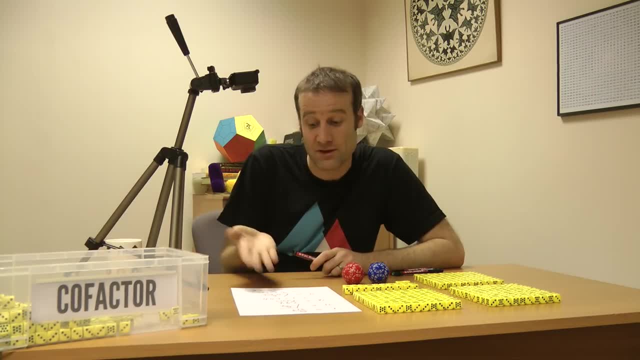 using this method, pi would be 3.12.. Even then, I still come a little way off that, so that's not great. More importantly, because this is a statistical method, the value you're getting out fluctuates. So, as I would have done this: 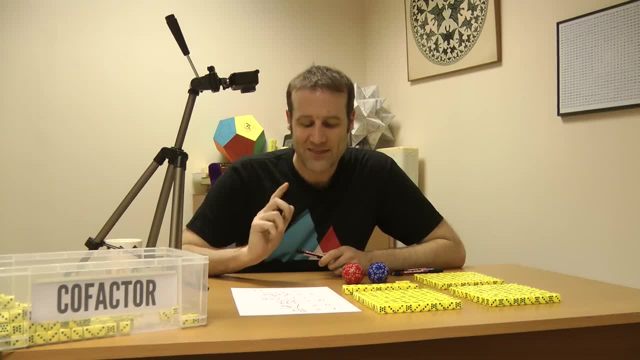 I'd be moving around the value of pi. That's actually why I was very, very deliberate at the beginning when I said I'm going to do 500 trials because the way you can cheat at something like this- not that I advise it- 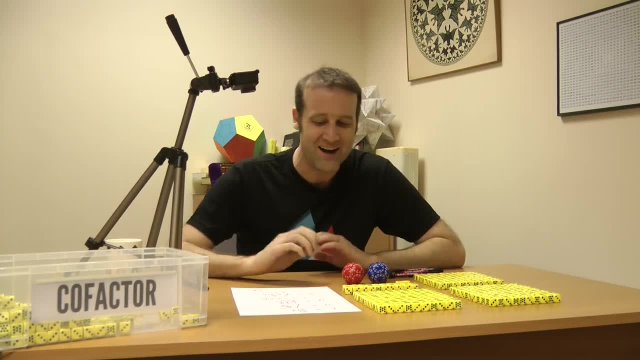 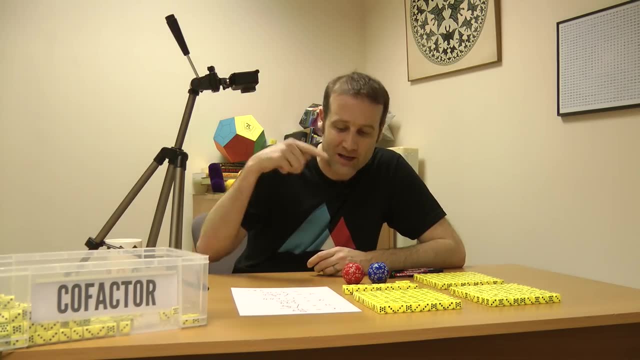 but if you want to cheat and make it look like you're better at this than you are, all you do is you keep track as you're going and your value. So if I'd been following my constantly updated estimate of pi for every single time, 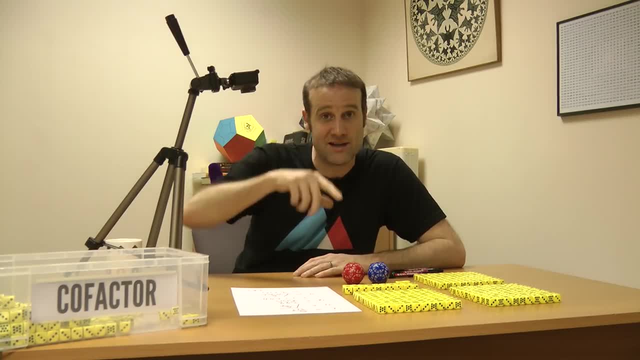 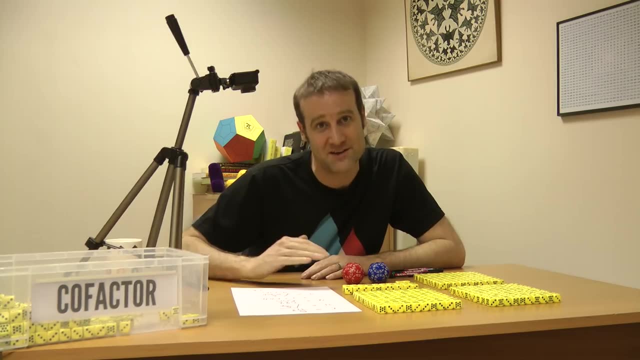 I categorized a pair of random numbers. I would have seen it going up and down. Occasionally it goes through pi, And so I could just stop. when it's one of the times it goes from being an overestimate to an underestimate, Stop bang on it. 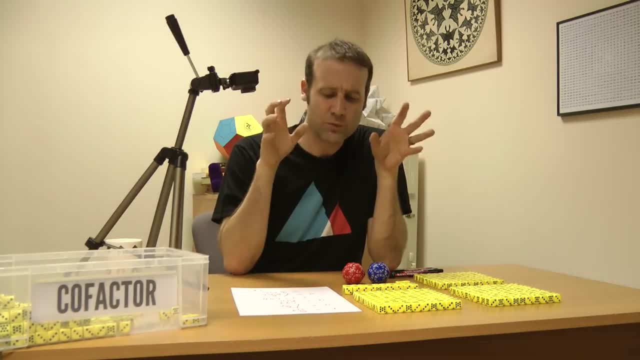 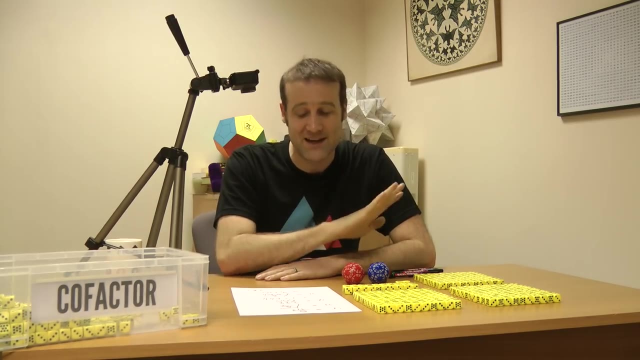 and get a disturbingly accurate value. Always be really suspicious. if people do something like this and they have a bizarre number of trials, They've probably stopped or only used the data that gives them a really accurate answer, Whereas I specified 500 pairs before I even started. 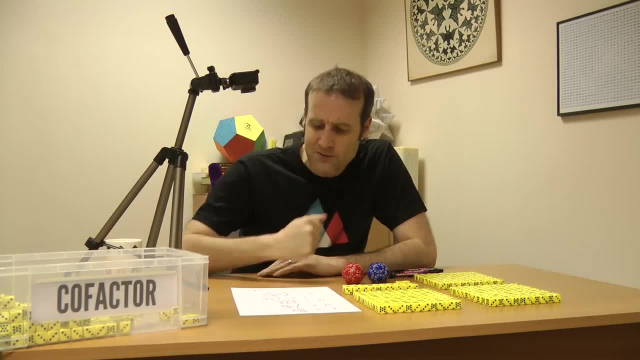 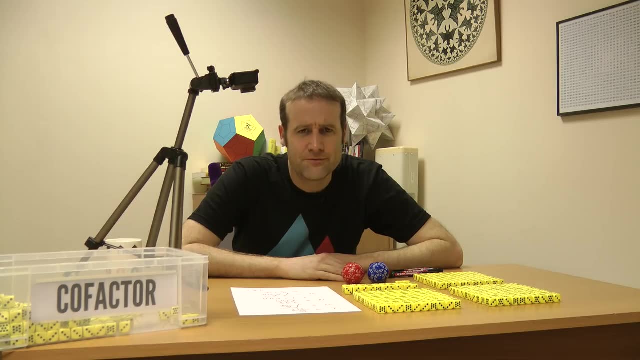 because I wanted to be genuine right, So I knew that's a genuine answer. I'm happy. within 3%. Come on, that's pretty amazing. Didn't I get something like 3.04 or 5 last year on Pi Day? 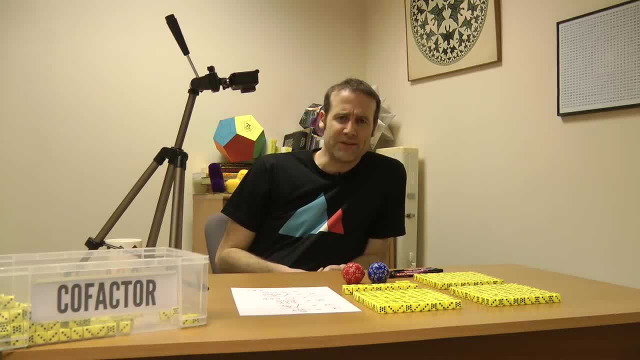 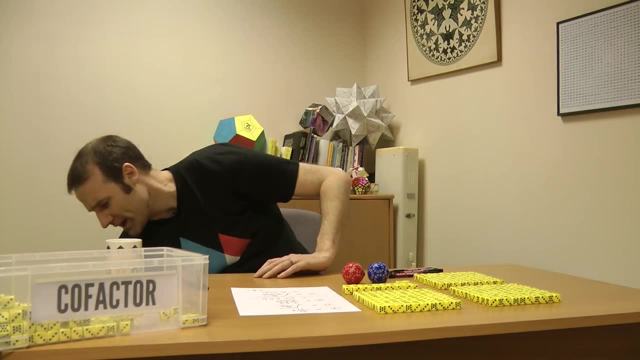 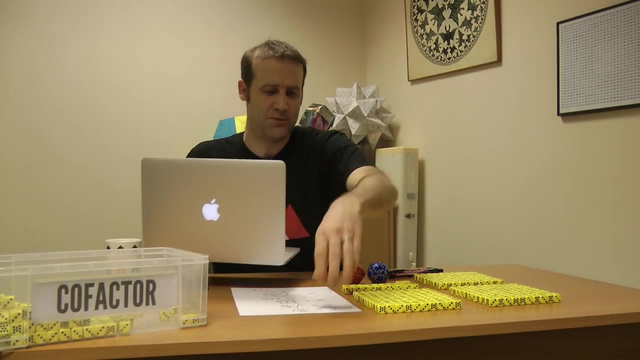 when I did it by hand. I mean, I am all about the underestimates. One last thing: if you want to try this yourself, you don't have to roll random numbers over and over again. You can cheat and do it on a computer. 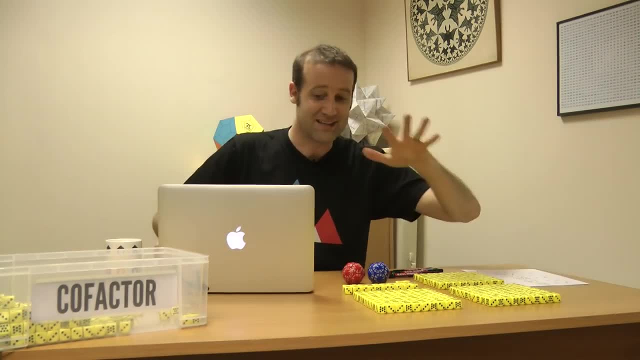 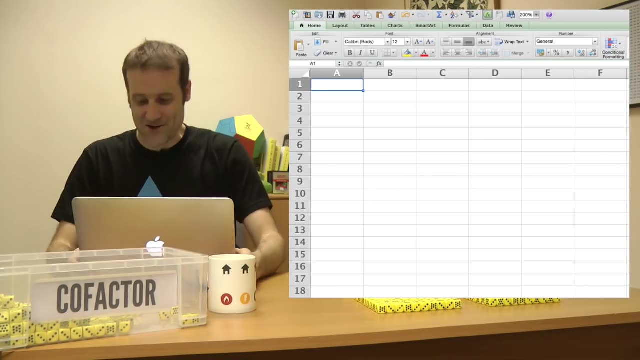 I'm now going to show you how you can simulate exactly the same thing yourself in Excel. Okay, you can see what I'm doing on the side over there. So Excel can give you a random number if you use the rand function. Open and close brackets. 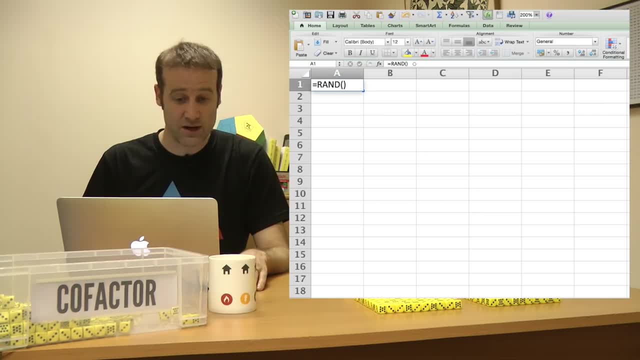 There's nothing you want to put in there. So there you are: 0.51, 0.98, and this is giving you a random number between 0 and 1.. We want a random number between 0 and well, if we're going to do these, 120.. 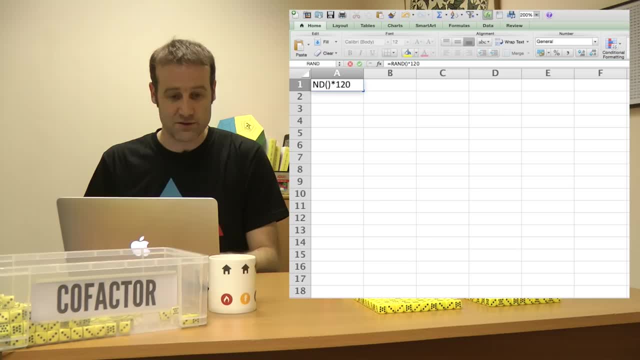 So what you do is, first of all, you multiply that by 120.. Now you're getting random numbers between 0 and 120. But you want a whole answer out. the other side- And this is a little pro tip here- You want to use the round up function. 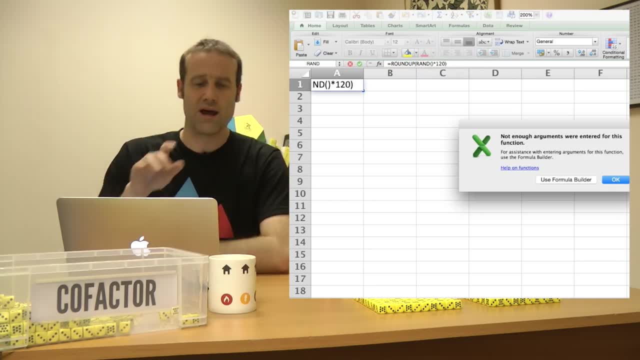 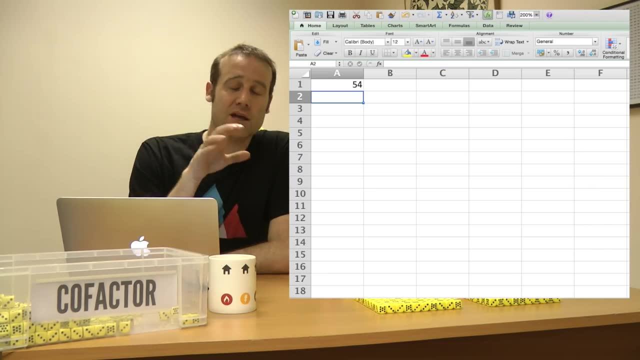 in Excel. If you just straight up round, you will not enough arguments. oh yeah, sorry, round up always forget no decimal places. If you just use the straight round, you'll get 0 and 120.. So you have 121 options. 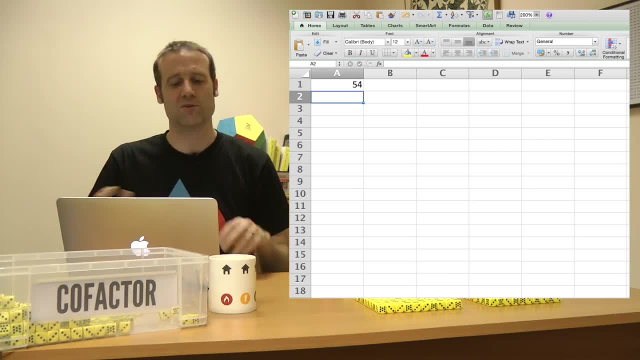 which are all equally likely, apart from 0 and 120, which are both half as likely as the others. If you round up, you get 1 to 120. Or completely fairly. So that's there's your formula for that. If you want to get excited, I guess. 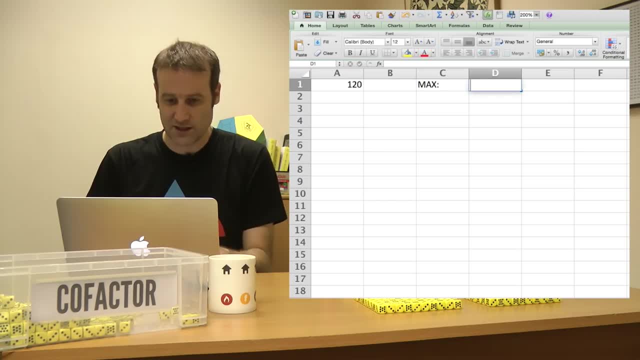 what we could have done is said: here's the max value, it's 120. And then, instead of putting that in there hard, we can say: it equals that one over there, But actually we never want that to change, So let's just lock that in place. 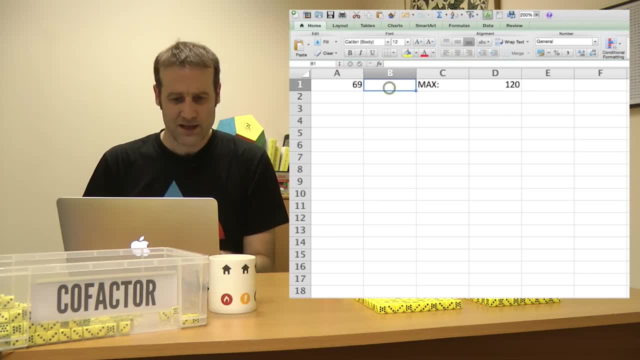 Okay, so there's our formula for getting a random number. Here is our second random number. Let's have a bit of space on the side here, And so, as you can see, every time I move we get a new pair of random numbers. 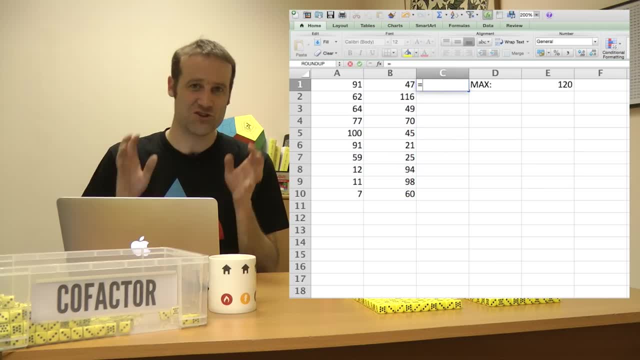 being kicked out. There's actually a function in Excel for the greatest common denominator. It's the GCD function. unsurprisingly, We want the greatest common denominator of the two numbers next to it. And there you is, That one's 3.. 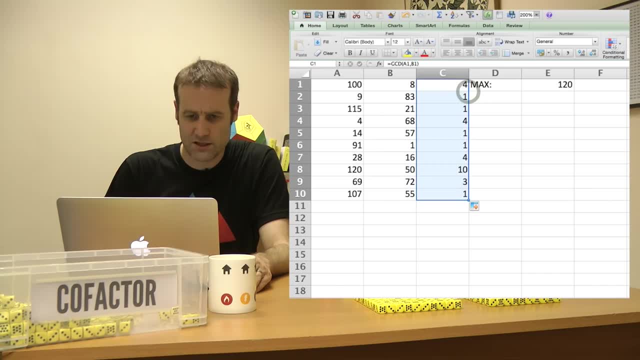 Oops, There you go. That one's, There you go. So that fills those in, And what we actually care about is if that greatest common denominator is 1 or not. So what you can say is: if the greatest common denominator equals 1,. 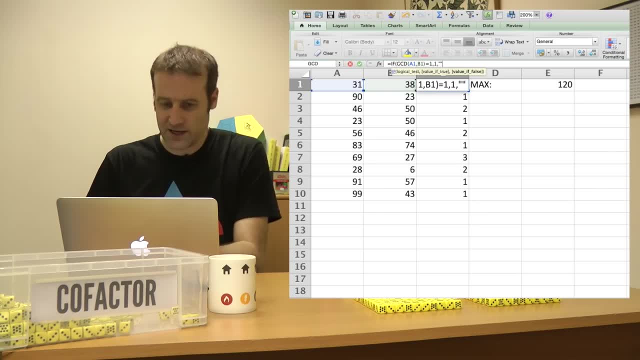 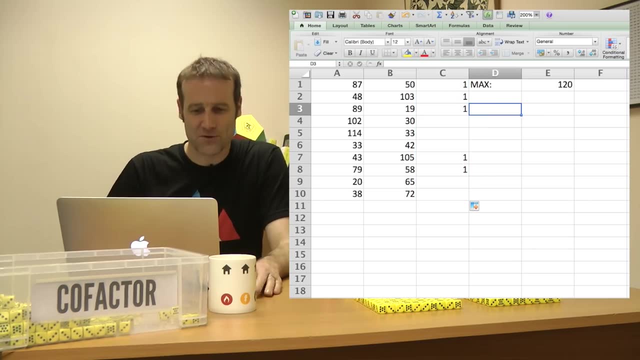 then give us a 1.. Otherwise blank. Okay, cool, And let's propagate that down. So okay, there we go. So now we only get a 1 if they are co-prime. You can see where this is going. 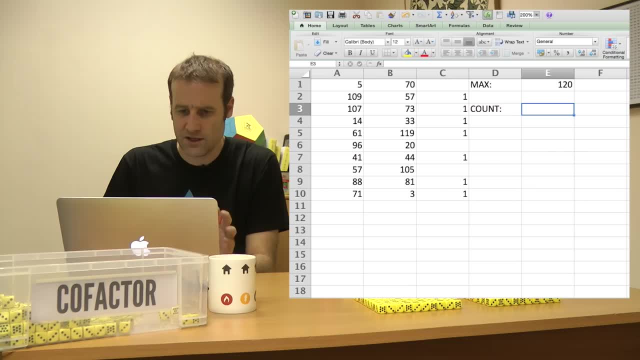 This is the count for how many are. co-prime, that is equal to the sum of those ones, right? So that counts how many of those. And then what we can do is say let's do this for the first. I don't know. 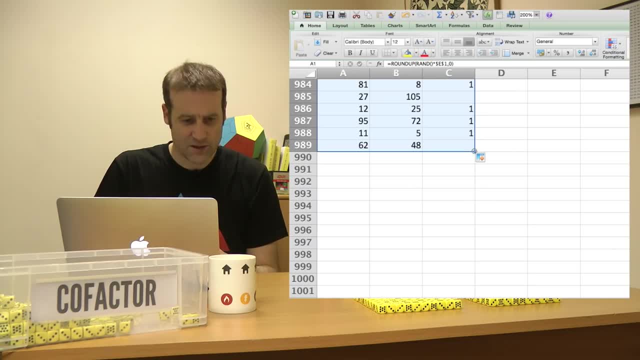 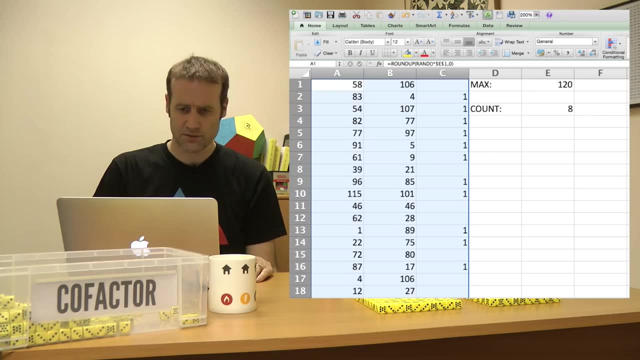 We reckon 100, 1,000.. Let's go all the way down to 1,000. So we're now doing twice as many as I did, which makes my achievement look a lot better all of a sudden. I'm quite pleased with that. 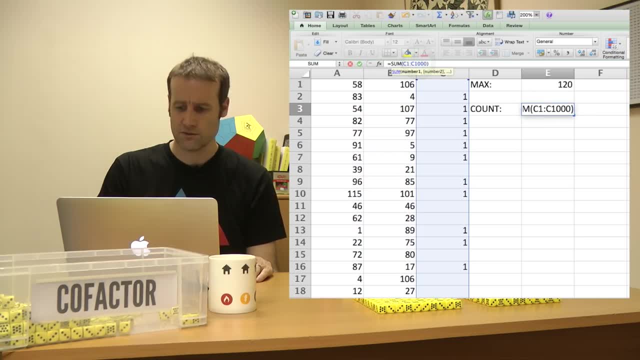 Okay, so then we now need to count. Instead of just doing 10,, we do 1,000.. So there you are. The first time I've run it, we had 599.. And 95 out of 1,000.. 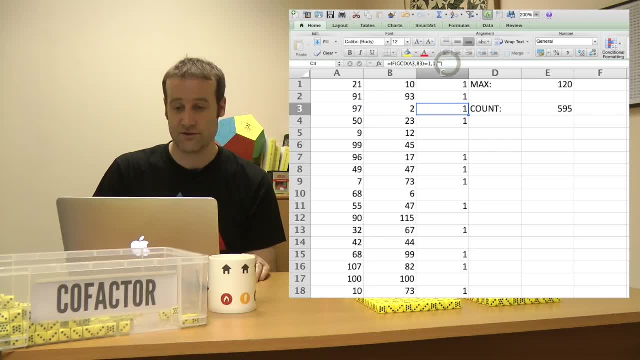 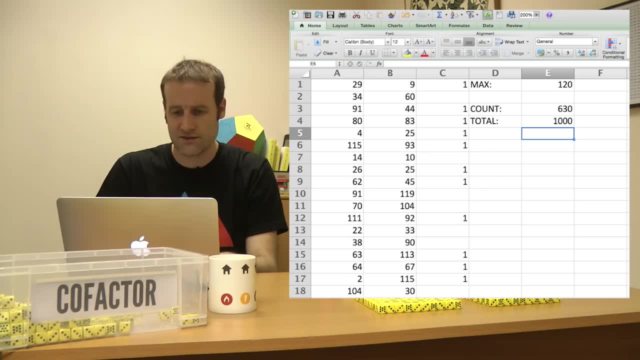 You could do a count function to get this. It's- Let's just say it's- out of 1,000, which means our probability is that divided by that. There you go. That was easy, Okay, and now? So that means that our pi estimate is. 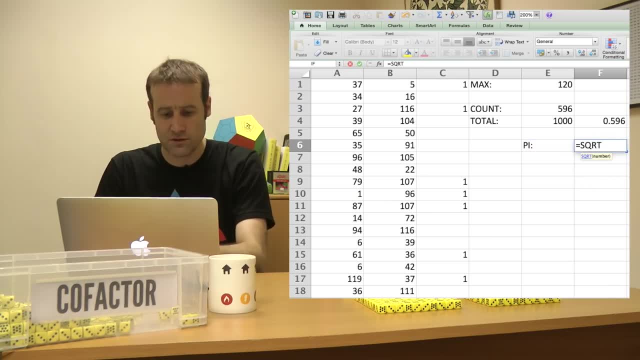 Equals: It's the square root of 6 divided by What are the probabilities? Pow, 3.24.. That's not bad 3.13, a lot closer: 3.13, again 3.07.. So this is. 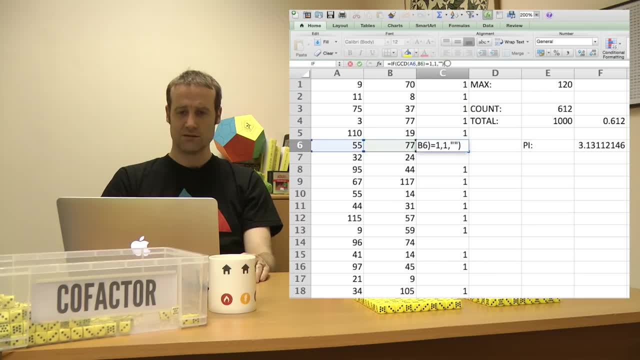 If I had done it for twice as long, these are the kind of estimates I'd be getting out for pi. In reality, like I said, the number of faces let us down, So let's crank this up to be a million. So now, if I was rolling two D1 millions, 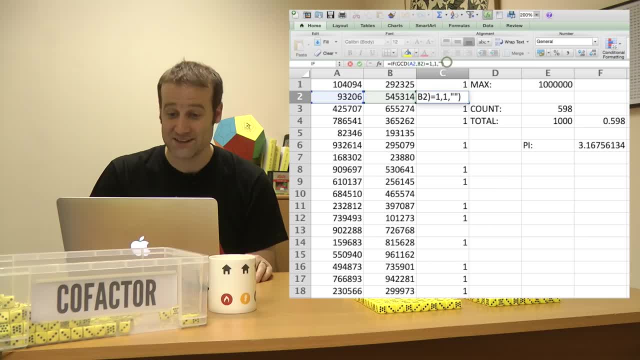 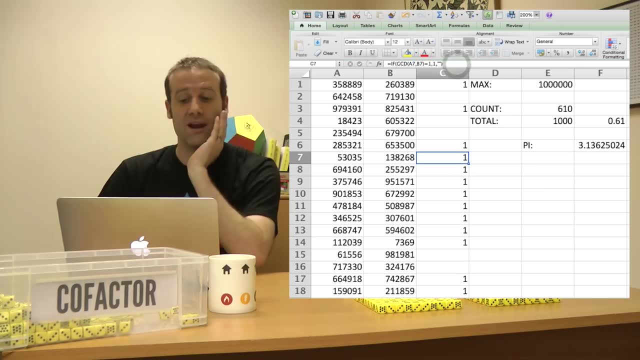 what kind of numbers would I get out the other side, 3.16. 3.07.. 3.13. 3.12.. Okay, closer, But still I think on average, if you check, they're coming in slightly under still. 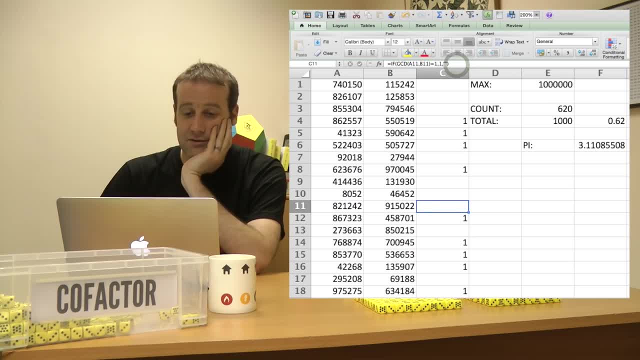 There you are, Oh, 3.24.. Okay, over, All, right. so now you can get the rough idea: 3.11.. 3.16. Right, If you wanted to, I mean obviously, you can program.